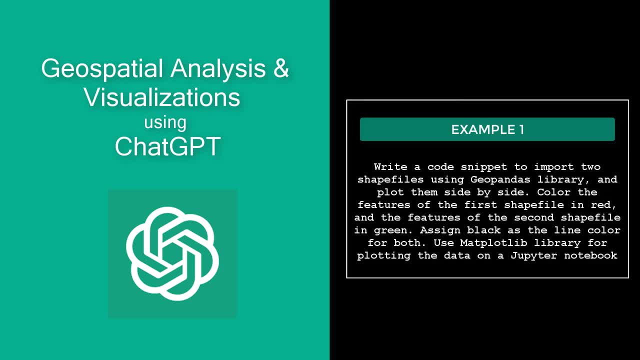 library. I'm asking to color the features of the first shapefile in red and the features of the second shapefile in green, And I'm assigning black as the line color for the features of both shapefiles. And at the end I'm mentioning that I would like to use the matplotlib library for plotting the 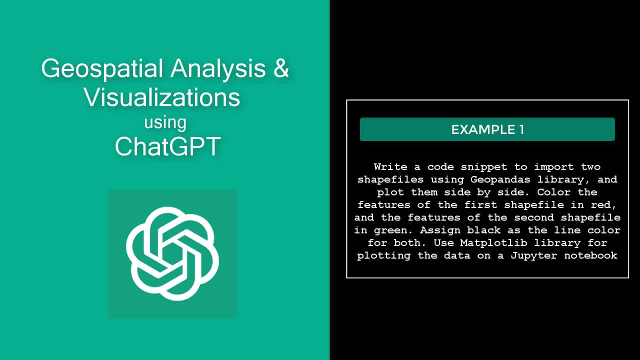 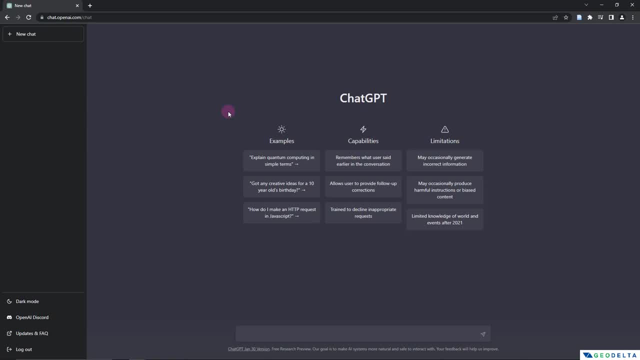 data on a Jupyter notebook. So let's just slide this request into ChatGPT and see how it responds, And this is the result. This is how the interface of ChatGPT basically looks if you're starting out for the very first time. If you head over to chatopenaicom, you will have to create a free account with OpenAI. 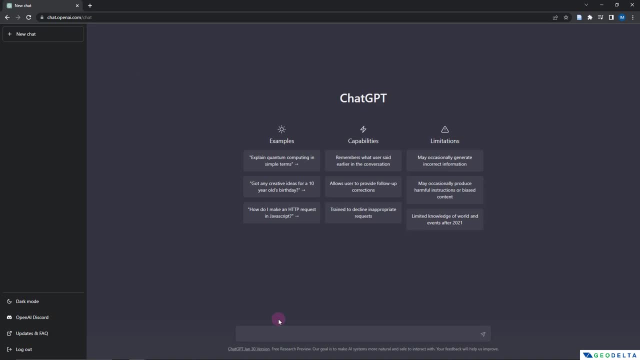 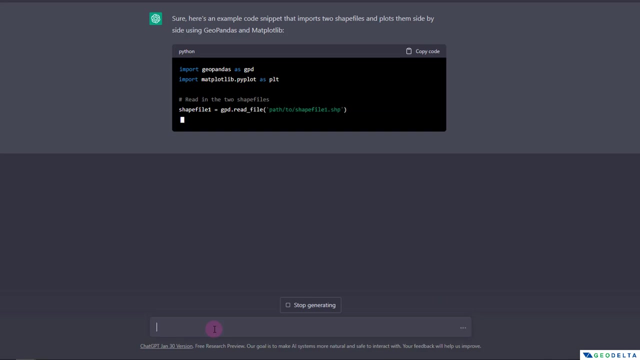 in order to sign up to use ChatGPT. So I'm just putting that request in right over here, And after that all we have to do is just simply hit enter And you can see that it's giving us an example code snippet using both GeoPandas as well as. 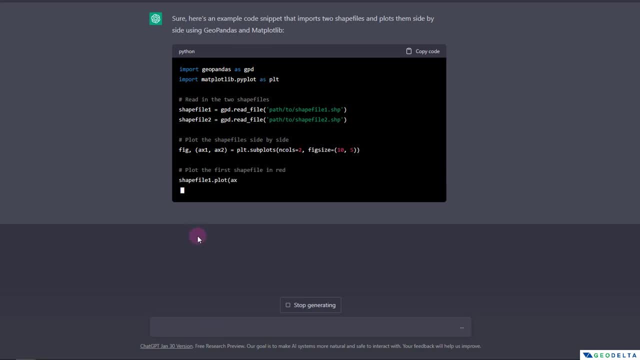 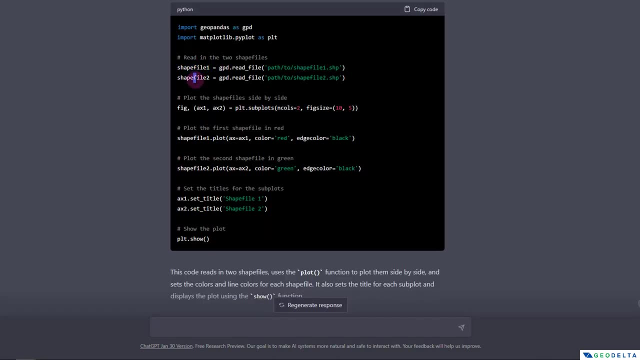 matplotlib libraries. So, as you can see, it's basically naming the shapefile one as shapefile one and shapefile two as shapefile two And assigning these sample names to the first and the second. shapefile was actually done by ChatGPT. That was not done by me, So it was actually smart enough to sort of assign a. 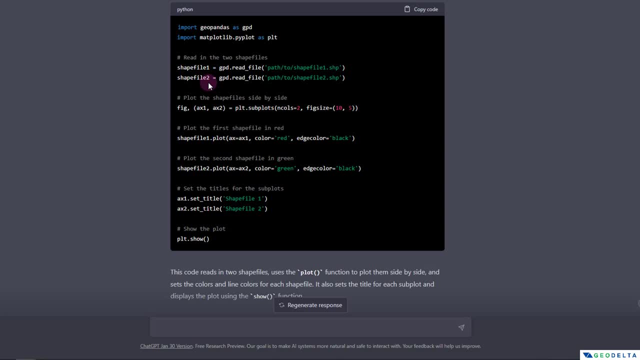 descriptive name in a way that the user would understand It's referring to when it's talking about an example code snippet, which is actually pretty amazing, And over here you can see that it's basically writing out the code to create a figure and access object And it's assigning a figure size right over here, which we would be. 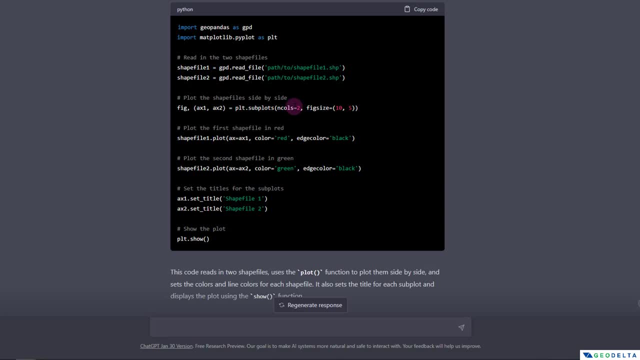 able to actually change if we wish to do so. And since I specifically mentioned that, I would like to plot these two figures side by side. it's basically assigning the columns value to be two, so that, with two columns, if you can imagine how a table looks with two columns, well, the two. 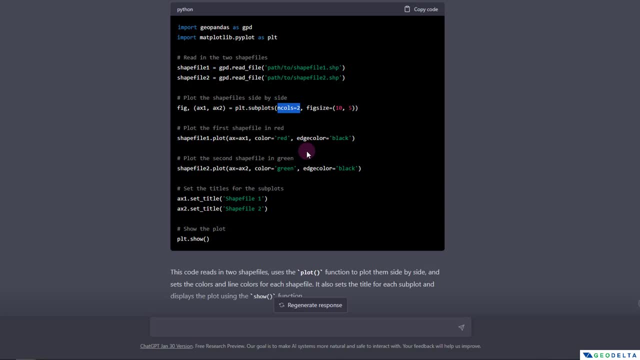 columns are going to be side by side. For example, if I want to plot a table of two columns, I can plot the table of two columns side by side, And if I want to plot a table of two columns, I can sort of structured side by side, isn't it? So that's the same. 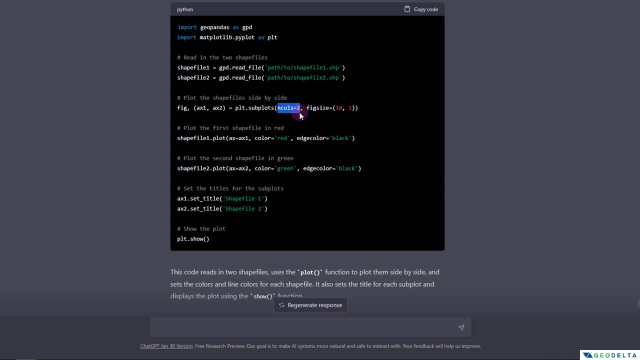 principle that we're using over here. So with two columns, we're intending to plot these two different shapefiles side by side, And it's asking us to use these two lines to basically plot the features: first one in red and the second one in green. 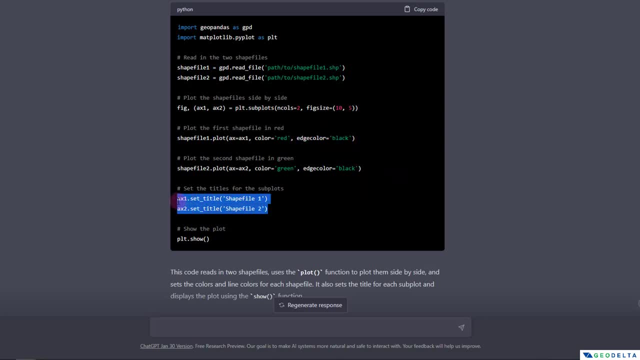 with the assignment of this edge color, And here's something that we didn't specifically mention. However, it was smart enough to understand that it would be a good idea to have two different titles for the subplots, So we can basically go ahead and 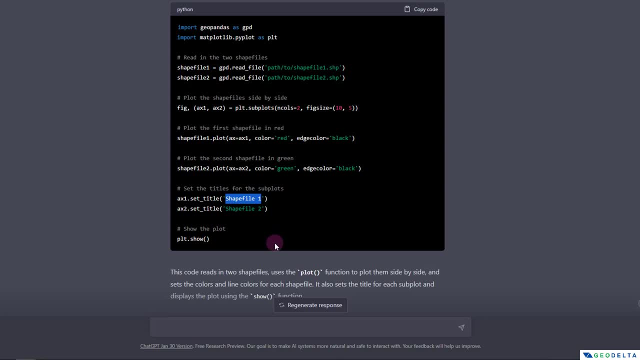 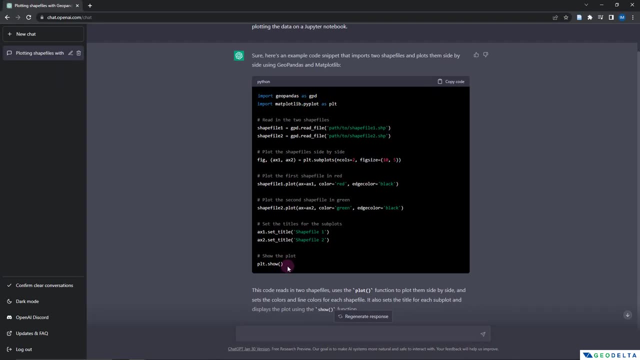 replace this part of the code with the title that we think is suitable. And finally, we can show the plot simply by adding PLT dot show. Alright, so what I'm going to do is I'm going to open up a Jupyter notebook first and navigate to your working. 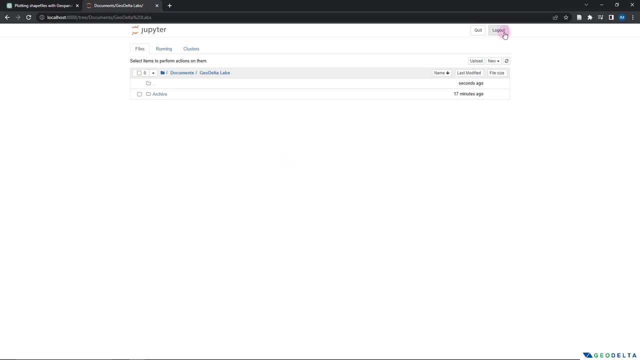 folder And after you navigate to your working folder in order to create a new Python script, what I'm going to do is I'm going to click right over here on the new. we can select Python, Python three notebook, basically Alright, now all I have to do is go. 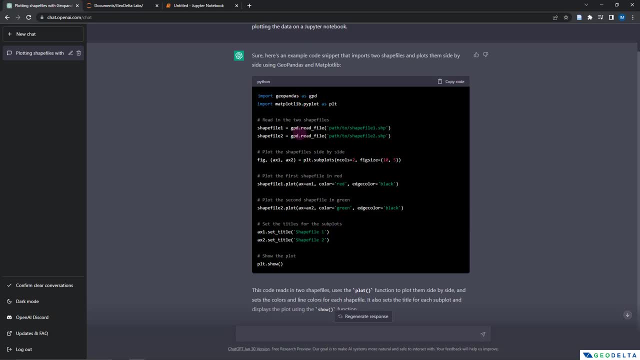 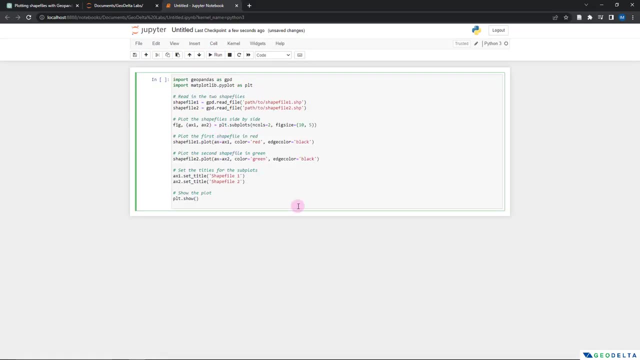 over here and simply hit copy code, which will sort of grab this code snippet onto the clipboard. head back to the Jupyter notebook: just right click and select, paste And, as you can see, we've got all the lines of code just in this. 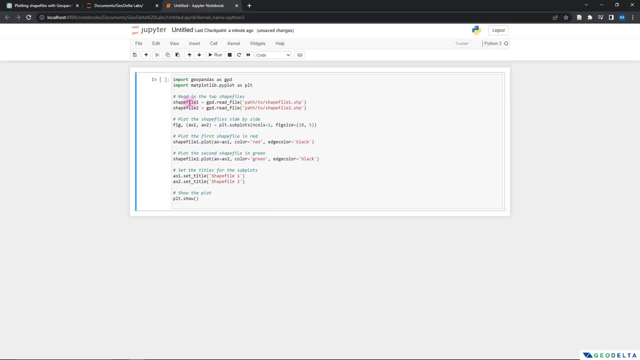 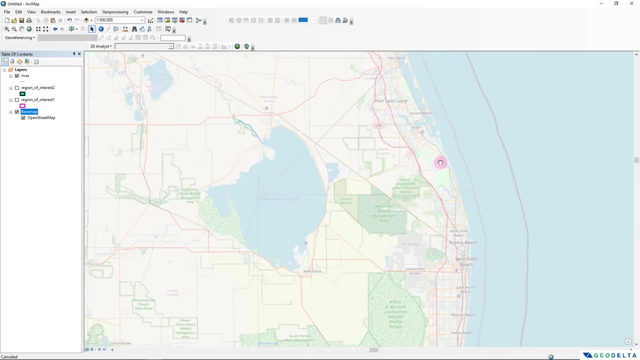 manner. Well now you might be curious: what exactly are we going to use as this shapefile one and the shapefile two? So, just for this example, I have prepared two different shapefiles. So here I'm basically opening up ArcMap just for the purpose of 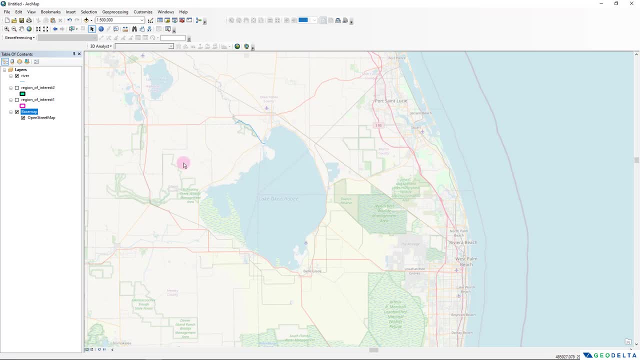 showing you guys what these two shapefiles are supposed to be. So I have two different shapefiles. So the first one is called region of interest one and the second one is called region of interest two. So if we quickly have a look at the 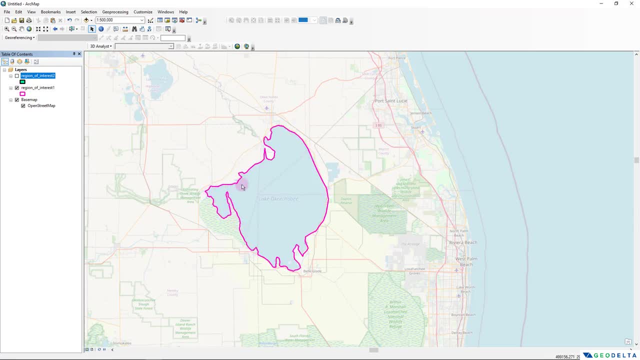 region of interest one. the extent of the region of interest one. it's basically a shapefile that encompasses this lake right over here, And if you would like to know the extent of the region of interest two, well, this is how the region of interest two basically spreads out. A part of it is: 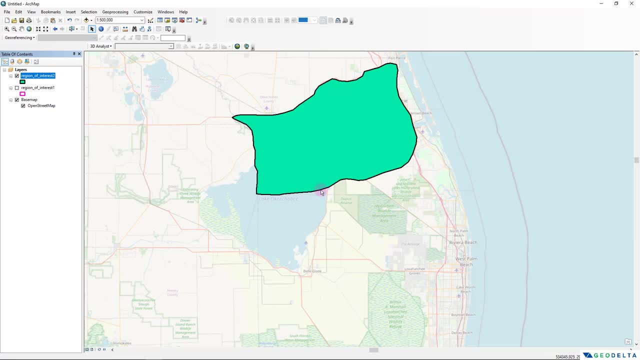 basically crossing over to the spatial extent of this lake as well. So this is just for your information, just so that you will have some sort of an idea what kind of shapes or what kind of polygons that we are dealing with when we import this into. 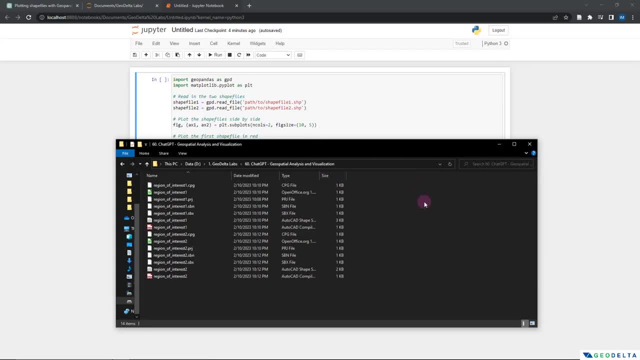 our Jupyter notebook later on And at the same time. if you're wondering about the, the actual files pertaining to these two different shapefiles, So over here you can see the, the set of different files which basically makes up the region of interest. 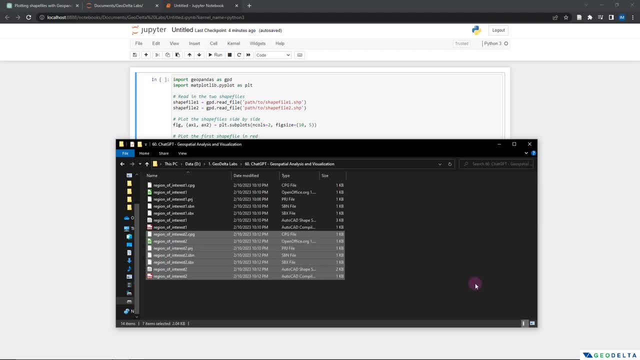 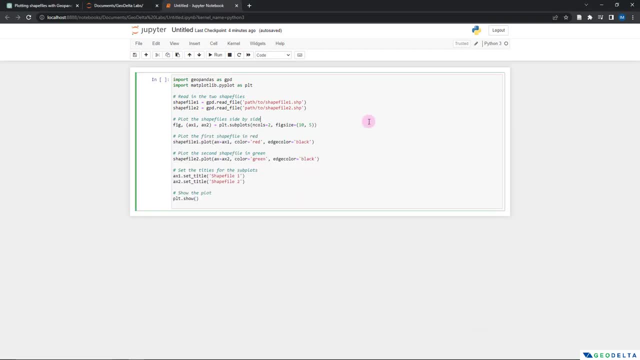 one shapefile And right over here, similarly, you can see the set of files which makes up the region of interest- two shapefile as well. Now, one thing to keep in mind is that when we are getting code snippets like this from chat GPT, chances are we 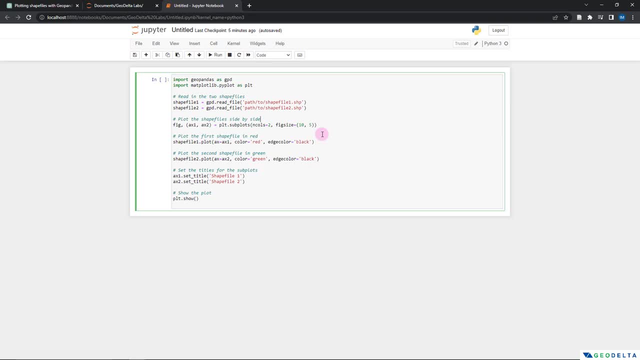 might not be able to execute this code immediately, because there's actual limitation when it comes to how much we can tell chat GPT- not that it cannot actually deliver, if you were to be very, very specific to the level where we also indicate the folder in which we keep our shapefiles as 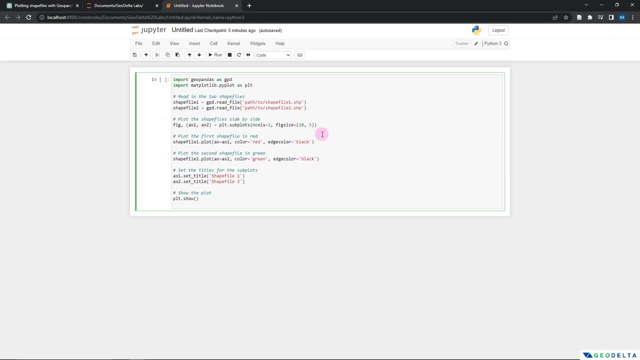 well, But I don't think it's not really necessary to be that specific, Because when it gives us a generic path like this, what we can do is we can basically replace this path or supersede this already given path by the actual part of the shapefile. 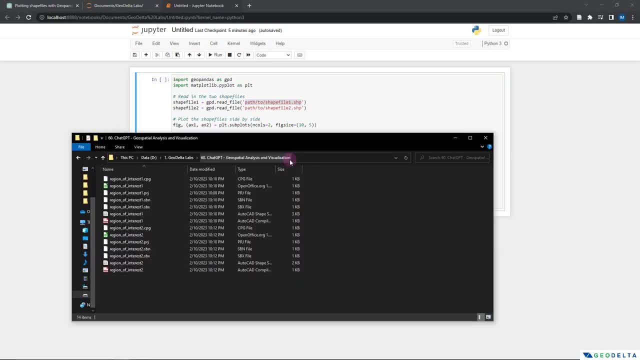 that we're supposed to use for our own analysis. So in this case, what I have to do is I have to copy this path and direct it to the region of interest. one shapefile, And similarly for the second shapefile I would. 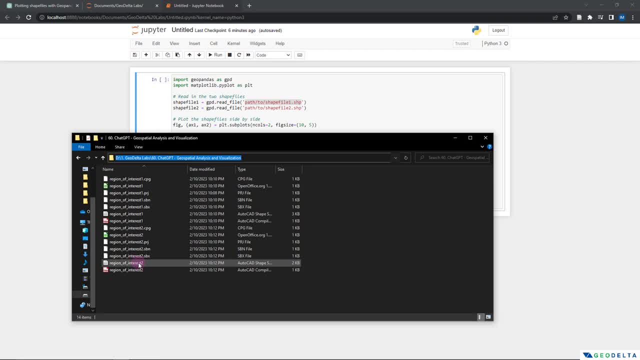 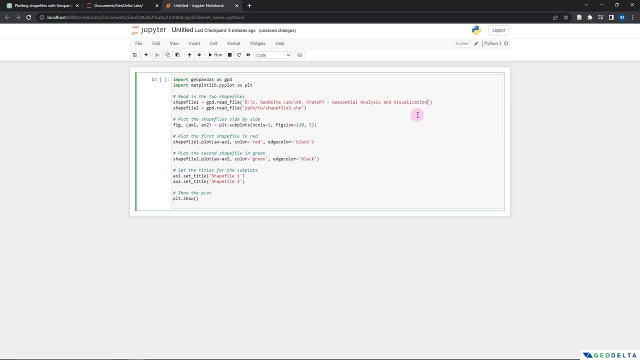 have to use this path and direct it to the region of interest to shapefile as well. So that's what we're going to do. So I'm going to replace this and add a backslash and name my first file as region of interest: one dot SHP. However, since I'm using 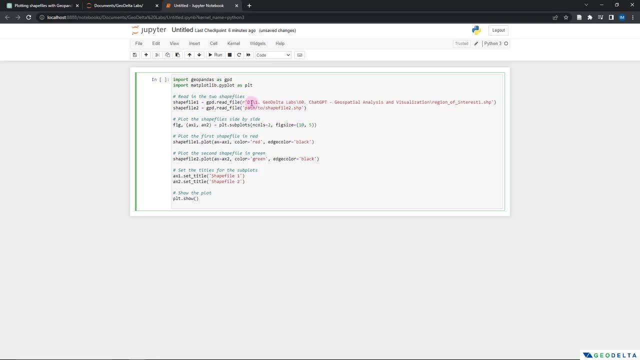 backslashes over here, I would have to add a simple R, or if you don't want to use this R, you will have to change these backslashes to basically slashes. But I don't want to do that, So I'm just going to retain this as. 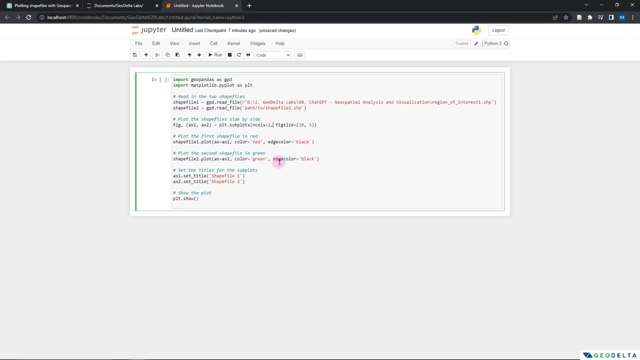 it is and just add simple R over here, So that it's. it's going to recognize that I'm referring to a specific path And similarly I'm going to copy this entire path and paste it over here. But for the second shapefile, instead of region of interest, one I'm 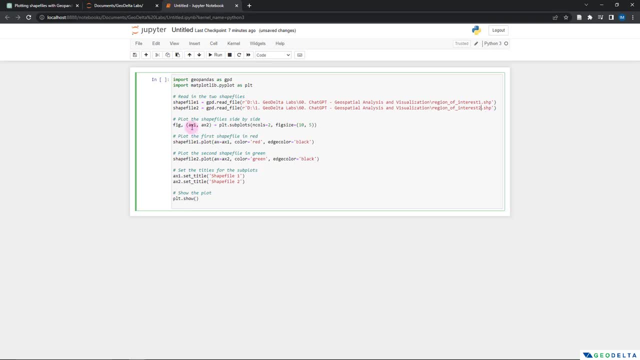 just going to add region of interest two And when creating the figure and the axis object. I don't really have any amendments that I would like to do, So I'm just going to leave this line of code as it is. I think we are good. 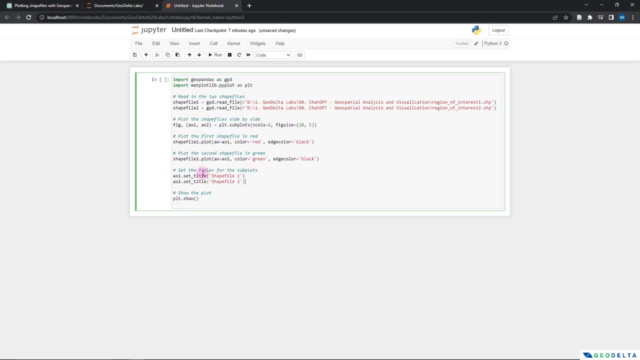 to go when it comes to these two lines as well, And just as the two titles. well, we'll just leave this shapefile one and shapefile two for the time being, And what we can do is we can basically do a secondary run and try to change these two titles, if you really. 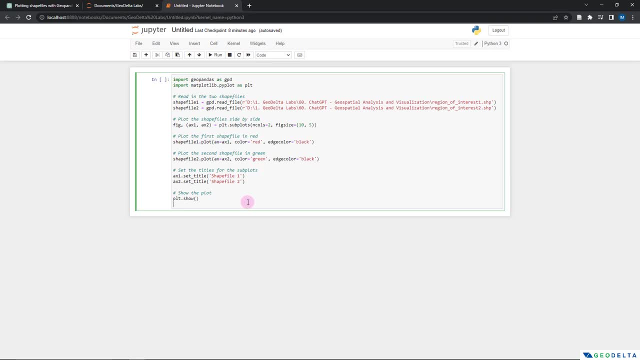 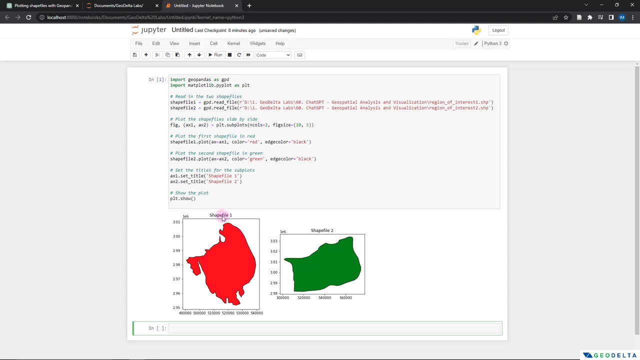 wish to do so. So the rest look good to me. And to test this out, what I can do is I can just simply click, run over here And just like that you can see that it basically displayed the shapefile one and the shapefile two side by side, exactly as we intended, And just. 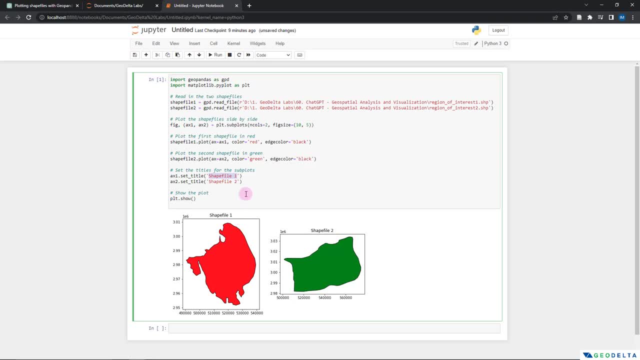 like what I mentioned, if I wanted to change the titles. well, I can simply pass a title called region of interest one, And for this we can make it to be region of interest two, And after that, if I click, run again. 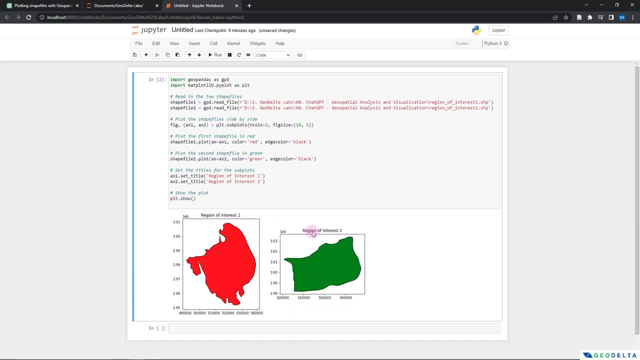 you can see that now. it basically displayed the two titles just like this, And over here on the x and y axis, what it's basically showing us is the longitude and latitude information, And this shapefile has a UTM 17. North projection. So these are the coordinates, basically. 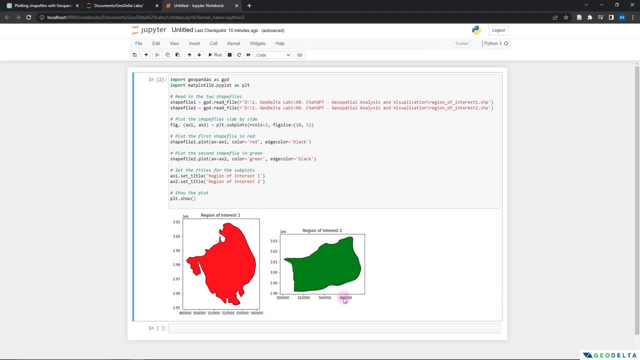 that are corresponding to that particular coordinate reference system. So it's pretty convenient to have those coordinate information displayed like this as well, especially if you want to know whether these two shapefiles are supposed to be spatially located far apart from each other or whether it's supposed. 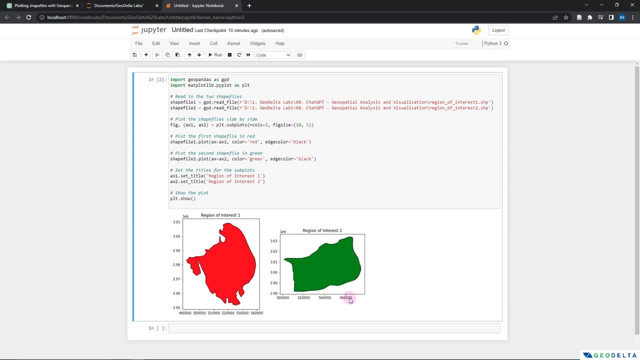 to be in the same region and whatnot. You can have an initial guess simply by looking at these numbers, whether it's basically falling on the same region or not. Alright, guys, so the next thing that I'm going to do is exactly that. I'm asking chat GP to amend this code that we have right over here. 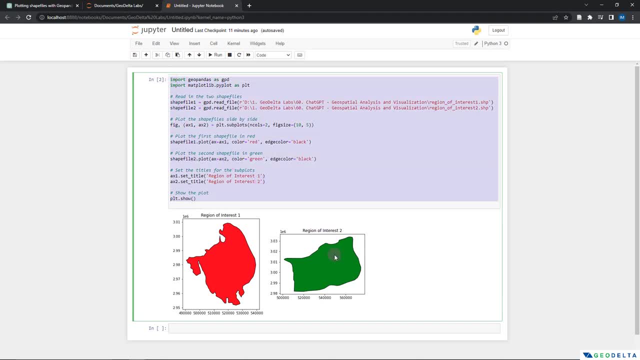 in a way that we plot the second shapefile on top of the first shapefile, just so that we can know whether it's really intersecting each other or not. Well, we already know that it does intersect, just because I showed you guys the extent of these shapefiles using ArcMap. However, let's just imagine: 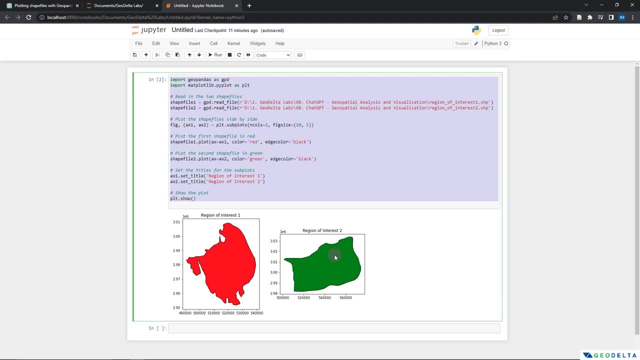 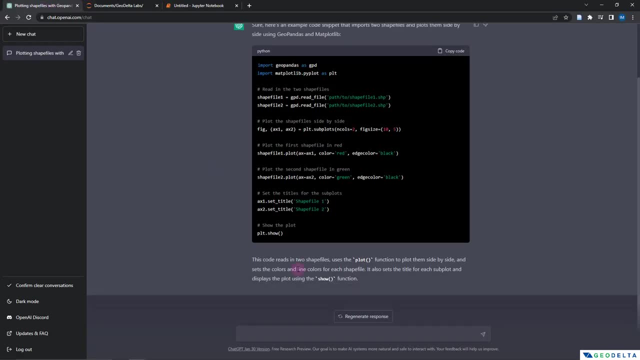 for a second that we didn't really pass through that step. We have no idea whether these two shapefiles are basically crossing over to each other's boundaries or not. So I'm heading back to chat GPT and I'm asking it, Alright guys. so I'm asking: how can I amend? 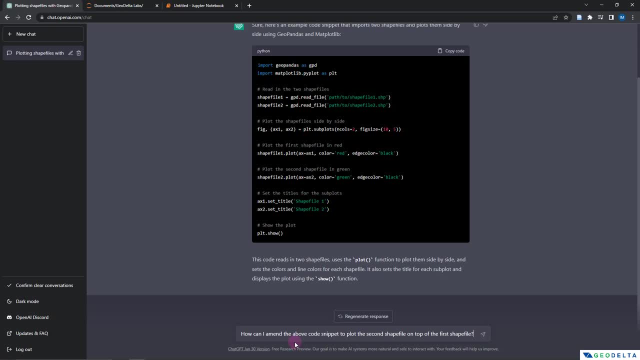 the above code snippet to plot the second shapefile on top of the first shapefile And we don't really even necessarily need to refer to the shapefiles as shapefile1 and shapefile2.. Chat, GPT is smart enough to understand, when we say the first shapefile and the second shapefile, that we are 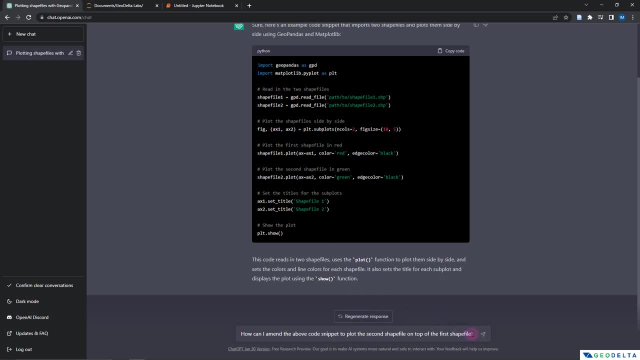 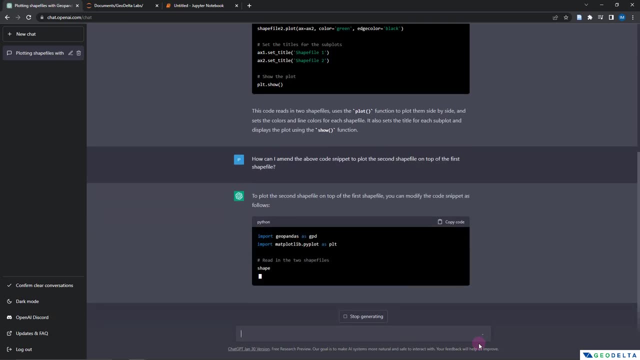 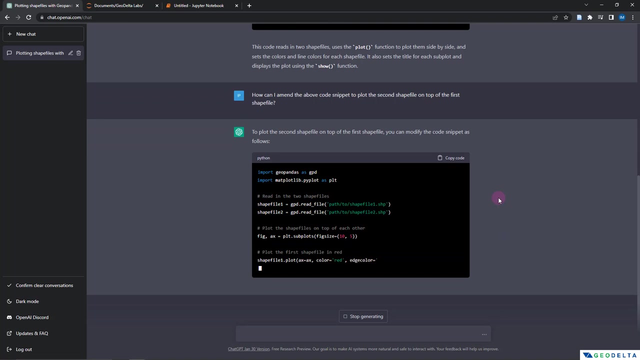 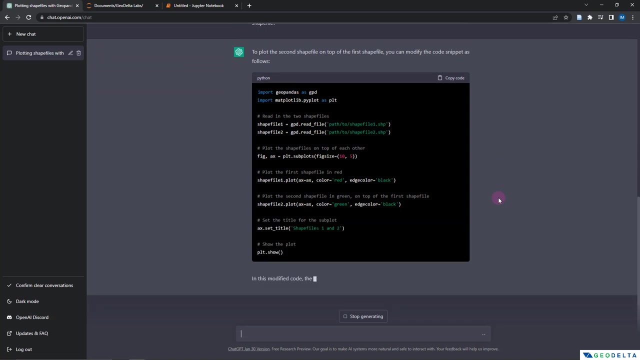 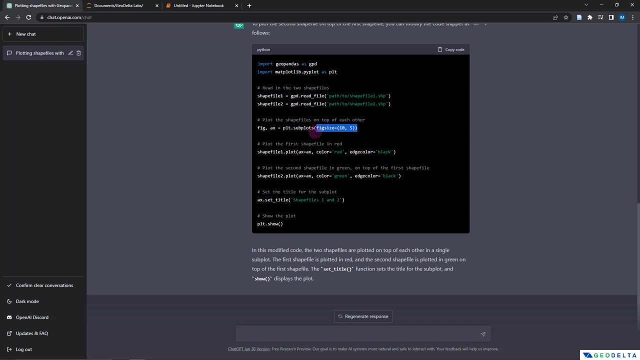 referring to these two in the correct order. So let's just hit and see what kind of a response we're going to get. So it's basically repeating the same steps that we had previously. So one of the key differences in the two code snippets is that over here we don't have that. 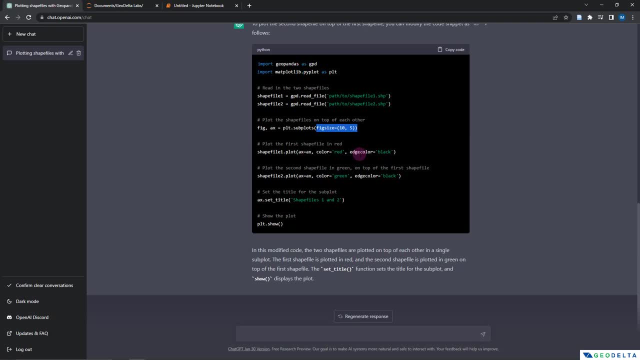 end calls argument, Because in this modified code two different shapefiles are basically plotted on top of each other in a single subplot, as it states right over here. So it's quite handy in the sense that it's basically giving us a lot of information about how to plot the second shapefile. 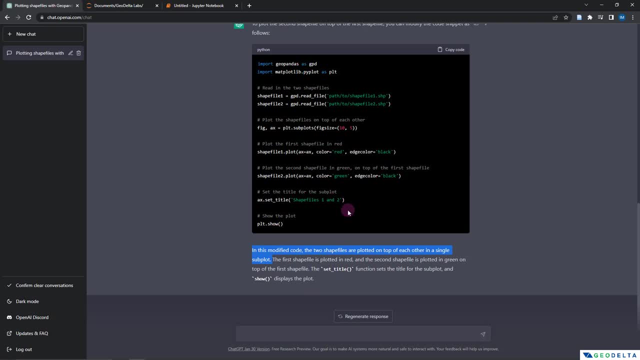 It's giving us a small description, following the code snippet, explaining what it has done. And, something quite important, when we plot the first shapefile and the second shapefile on top of each other, we no longer can assign two different unique titles. So in that case, 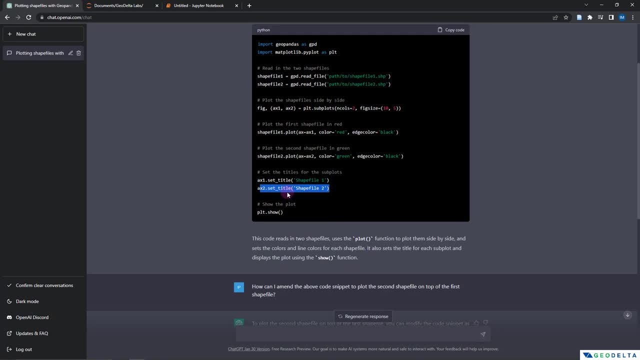 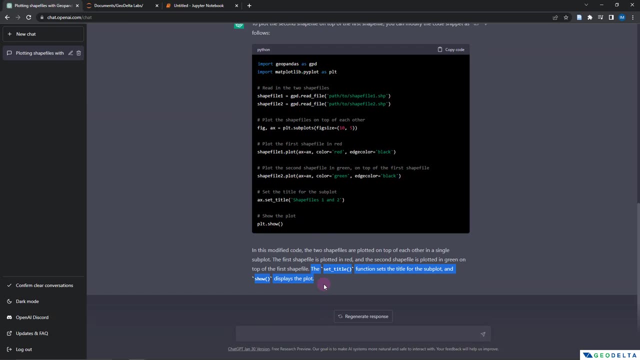 you can see that it got rid of one of these axsetTitle lines of code And over here it's basically justifying the reason for that, because now we're going to set a common title instead of just setting two different titles for the two different shapefiles. 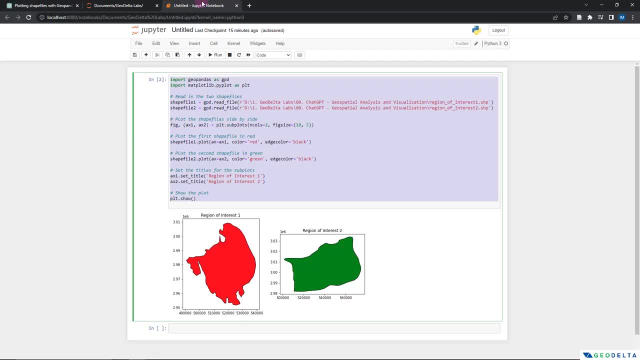 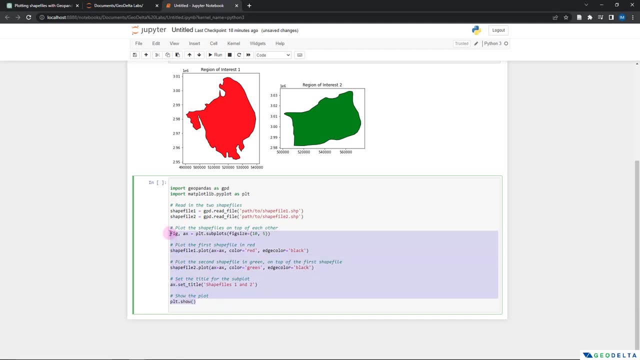 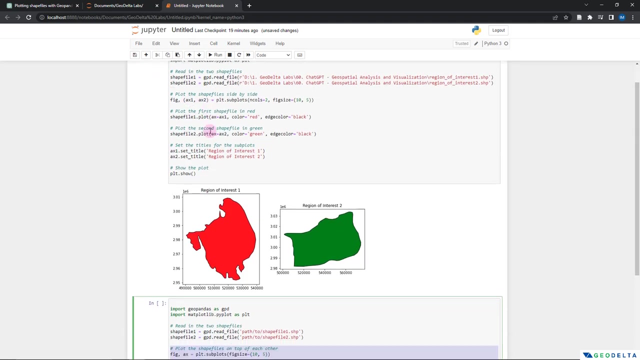 Well, what I can do is I can basically copy this code and I can paste it over here temporarily. And I think what I can do is I can basically copy this entire part, especially considering that over here we don't have the axis one and axis two, just like what we have right over here, because now we 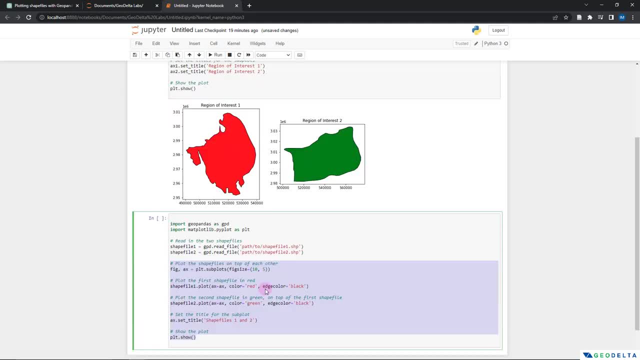 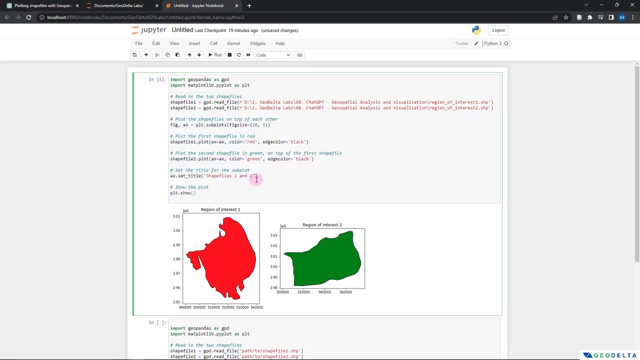 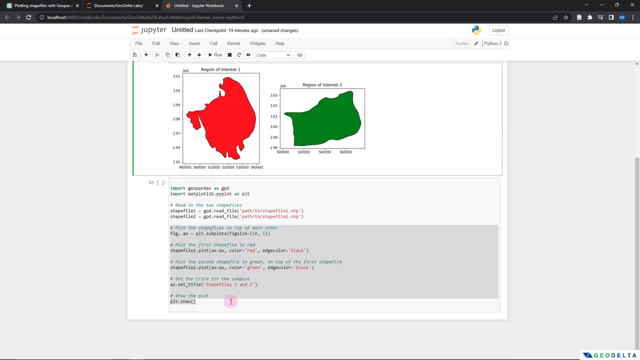 are plotting everything into the same plot. So just copy that part out And what we can do is we can just replace this whole thing. So anything that we think it's going to require an amendment, I think we can change the title over here And I can just simply hit delete to get rid of that code snippet And as a 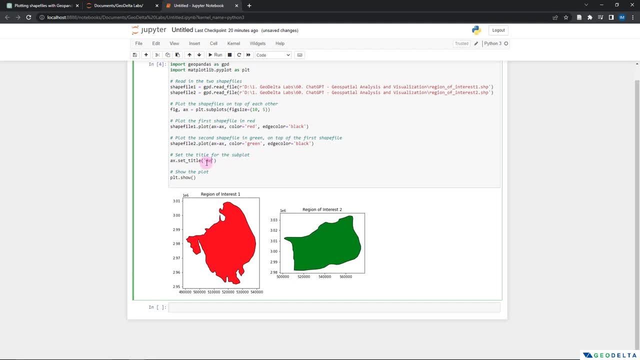 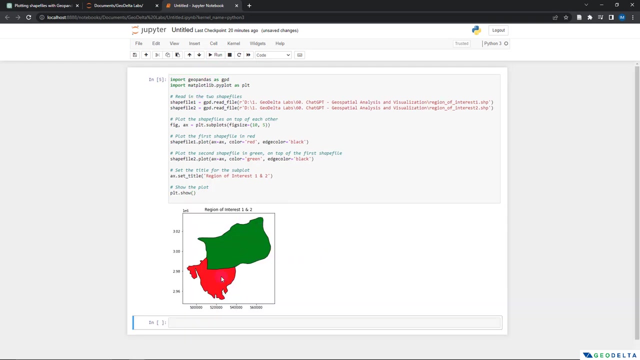 title. I would like to pass a title called region of interest one and two. Alright, now what we can do is simply run this code snippet and see how it looks, And, just as we expected, we can see that it basically plotted the shapefile two or the feature of the shapefile two on top. 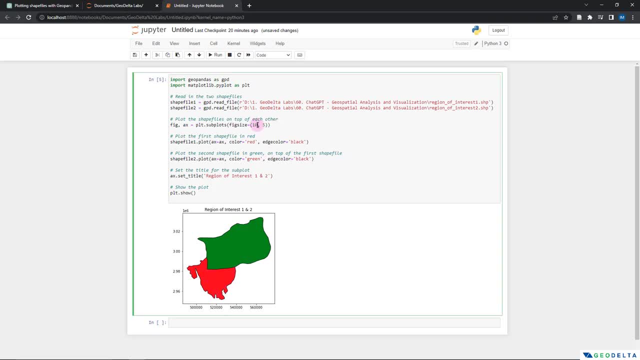 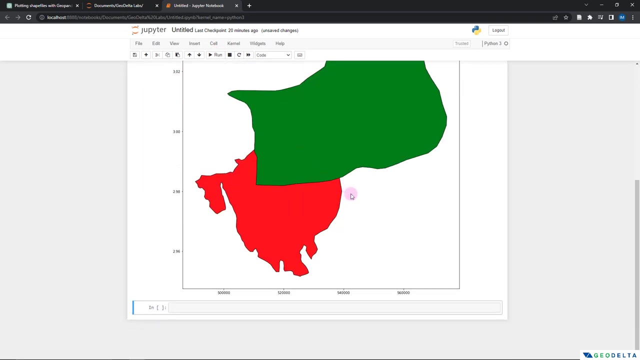 of the feature of the shapefile one, And we can always play around with the figure size, As I told you guys. let's say, if you wanted to make this to be 20. And this to be about 15. We can rerun the command And now you can see that it's basically expanding the. 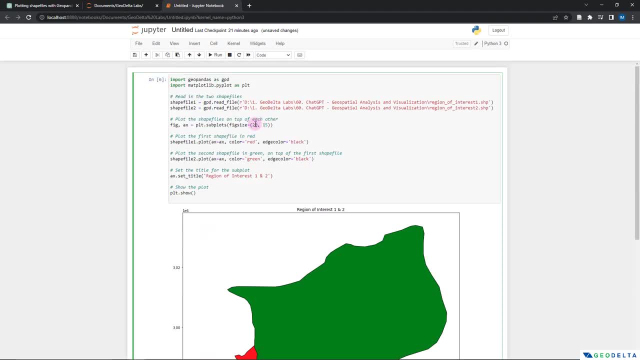 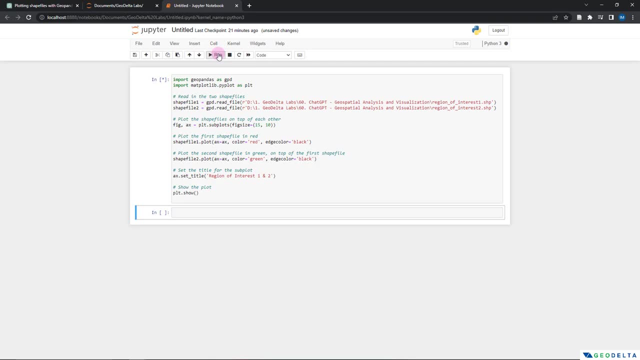 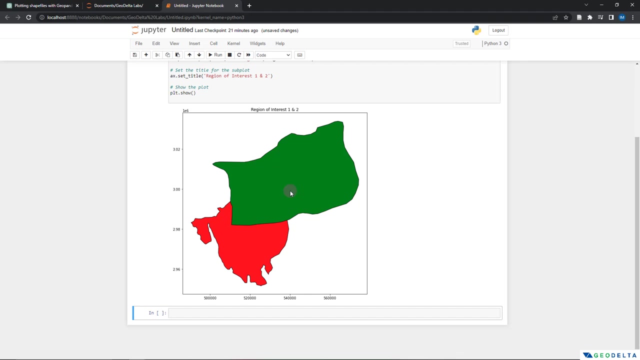 extent. Well, I think it's a bit too big. Let's set this one to be 15.. And this one to be about 10.. Yeah, I think this is good enough for me. Now, before I move on to the second example, I'm also going to do an additional. 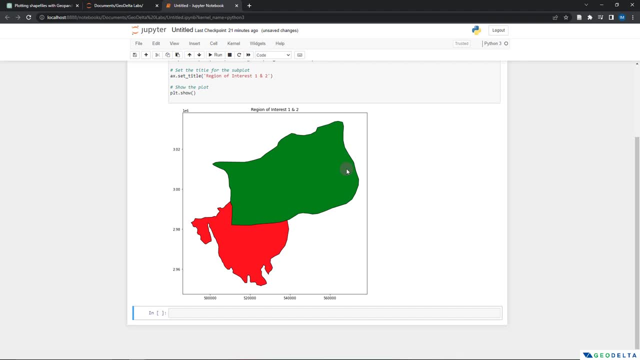 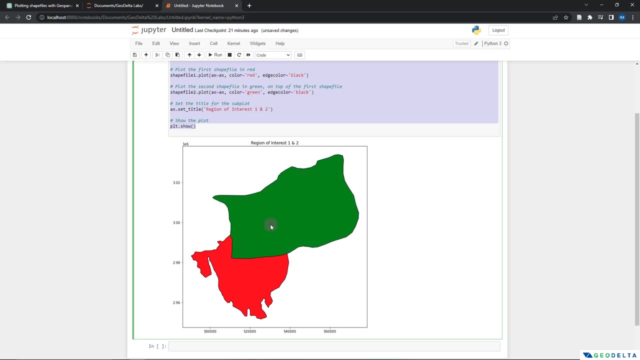 step And I'm asking help from chat GPT to amend this code further in a way that we change the transparency of the shapefile two just so that I could see shapefile one behind that, And that'll give me sort of an idea about the extent of the shapefile. 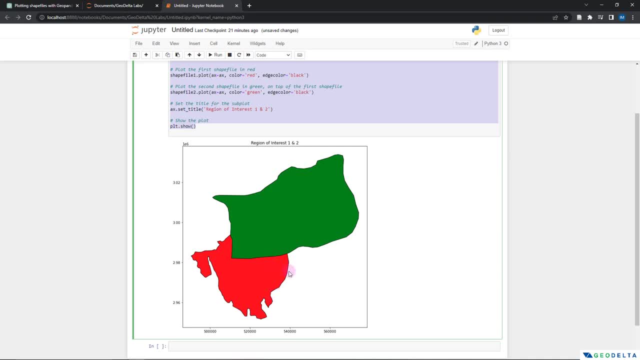 Of the features of the shapefile one, because when we plot the shapefiles on top of each other, I have no idea what is the spatial extent of this red color feature in its northern part, because it crosses into this green color shapefile And it's basically completely obstructed. 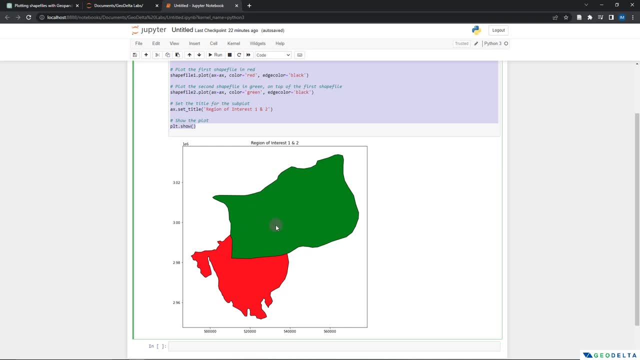 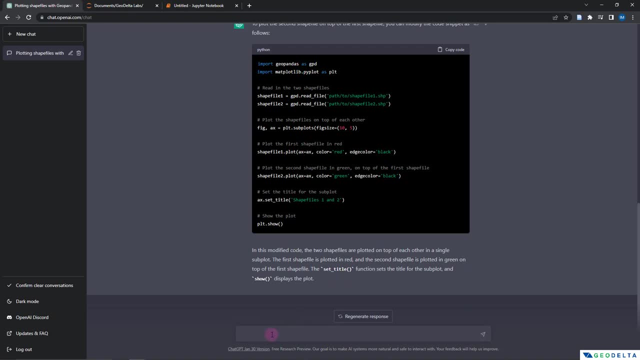 by this fill color. So I would like to increase the transparency of this shapefile two. So what I'm going to do is I'm going to ask chat, GPT the directions to increase the transparency of the second shapefile. So how can I increase the transparency of the second shapefile so that I could visually 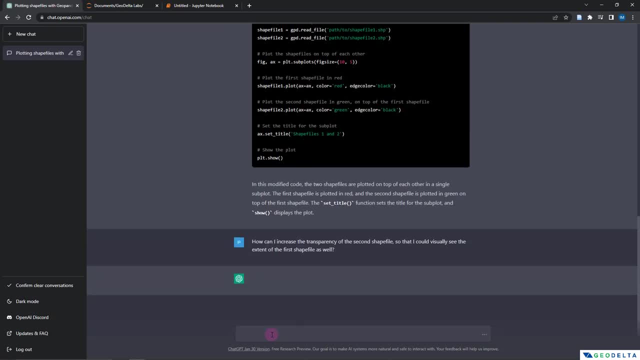 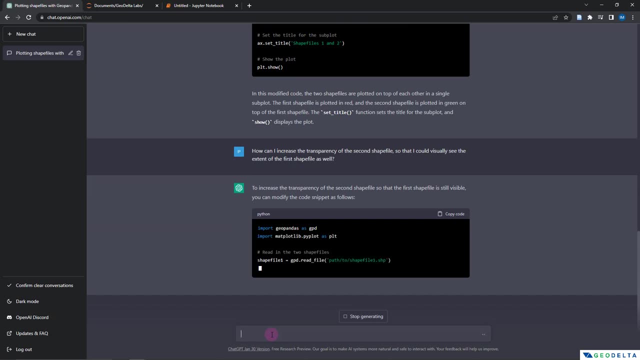 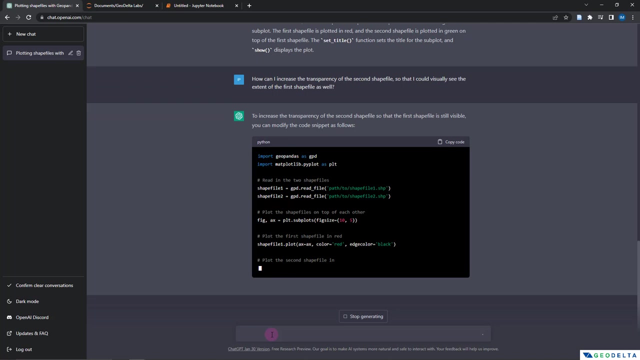 see the extent of the first shapefile as well. Okay, so let's go ahead and create a new shapefile. So let's go ahead and create a new shapefile. Okay, so let's go ahead and create a new shapefile. 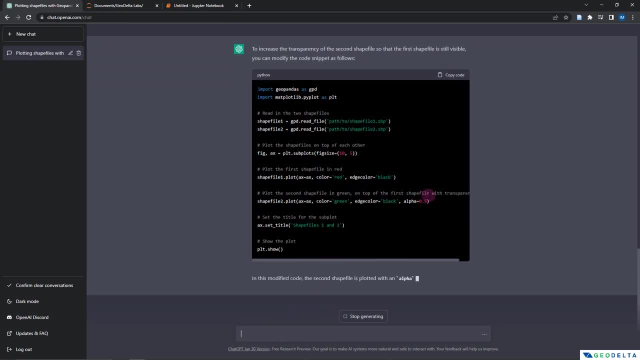 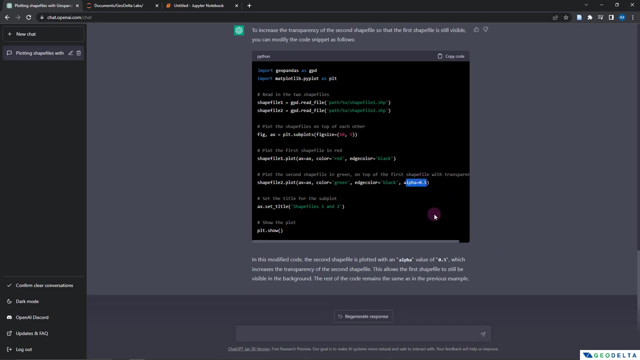 Okay, so let's go ahead and create a new shapefile And just like that, you can see what it actually added Additionally compared to what we had before. it basically passed this argument called alpha, which basically controls the transparency, and, sure enough, it didn't really forget to emphasize on that particular change. 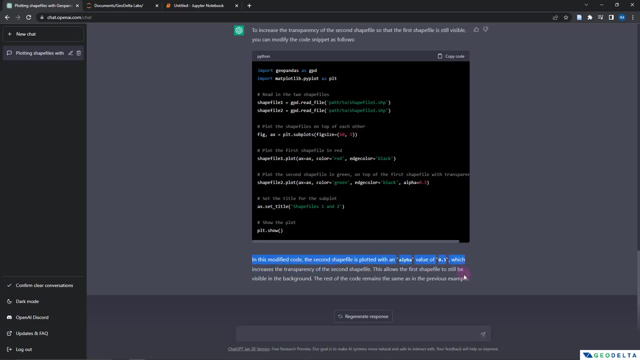 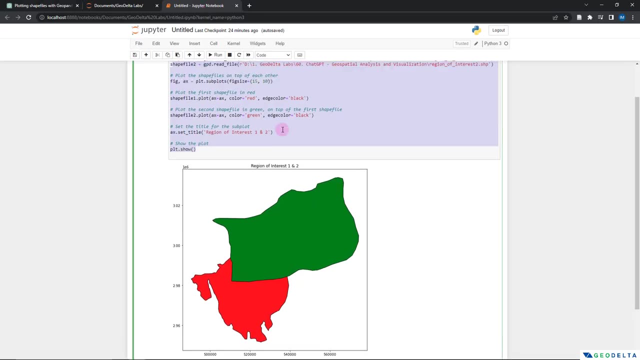 right over here as well, just so that we would know exactly what kind of a change that we are supposed to do. So I'm just going to copy this: alpha equals 0.5.. Basically pass it as an argument right over here. rerun the code. 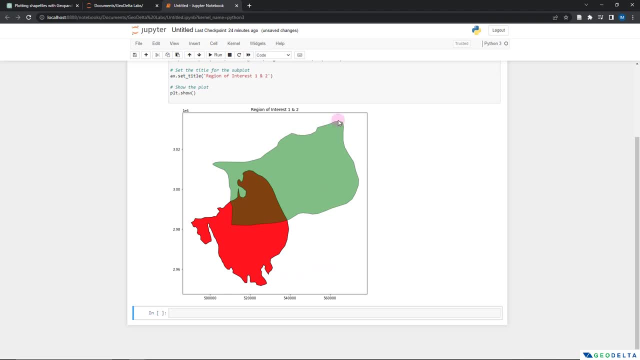 And, sure enough, we can see that the transparency has increased And now we could see the first and the second shapefiles and the common region where intersects each other, which is supposed to be this area right over here, All of these lines of code. we're actually able to find it if you were to do a simple. 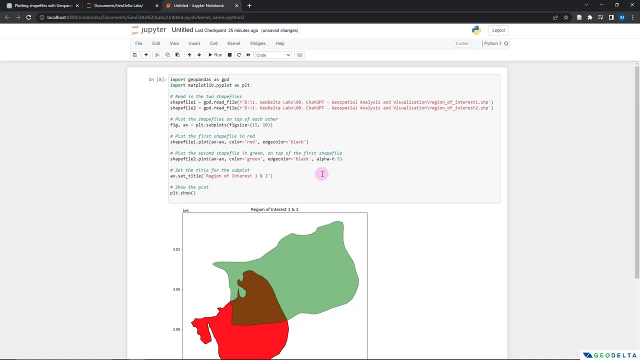 Google search. However, what's going to be very efficient when we use chat GPT as a tool that can increase our productivity. The first example is that we can be very specific in what we need, And it can save a whole lot of time that we otherwise would have spent just reading unrelated stuff on the internet. 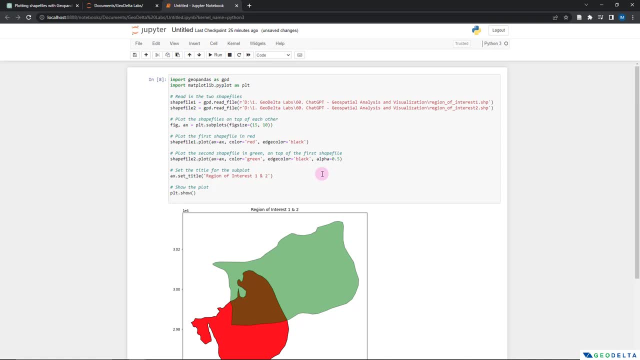 just to get to the point that we're trying to make. But when using chat GPT, we can be very specific to the T and it can guide us in the right direction without having to spend a whole lot of time doing unnecessary and unrelated things. 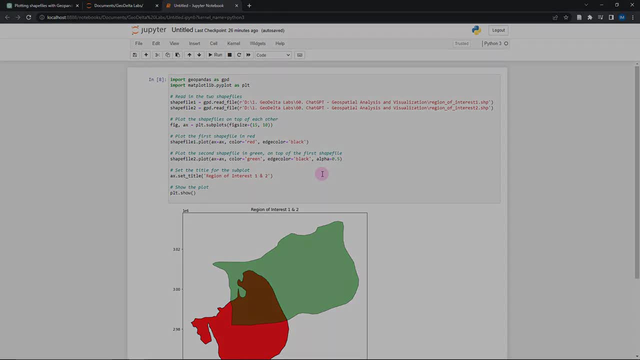 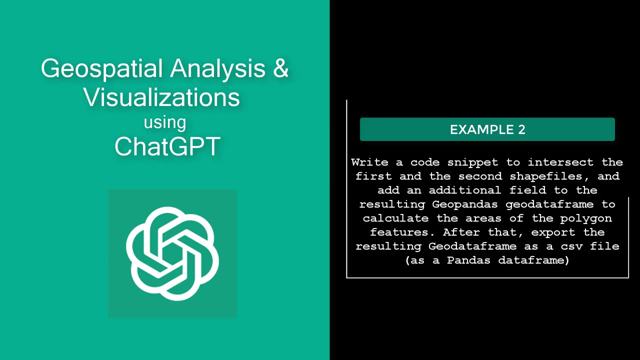 All right with that. let's move on to the second example, Example number two. So in the second example I'm asking chat GPT to write a code snippet to intersect the first and the second shapefiles and add an additional field to the resulting Geo pandas geo data frame to calculate the 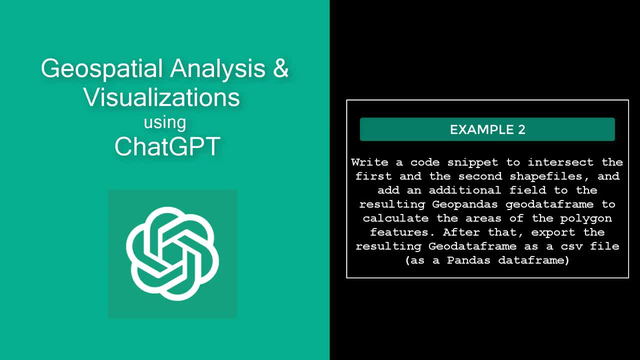 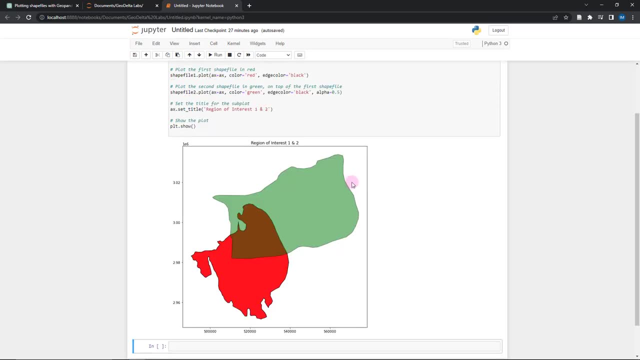 areas of the polygon features. After that, I'm asking chat GPT to export the resulting geo data frame as a CSV file or as a pandas data frame that we can basically open up using notepad or Microsoft Excel or a software like that. So if you come back to the plot, 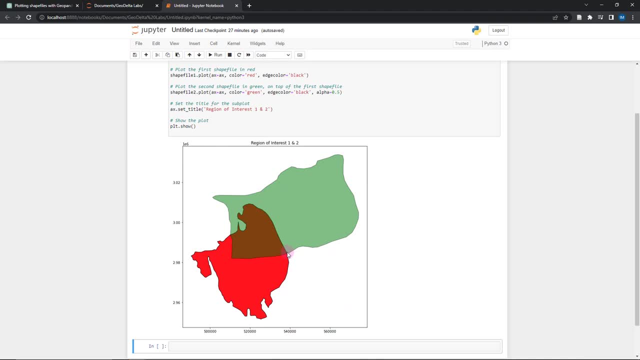 you can see that we have this region of interest or the, or this common ground that belongs to both region of interest to, as well as region of interest one In the second example. what I'm asking, chat GPT, is the line of code that we need to use to basically intersect these. 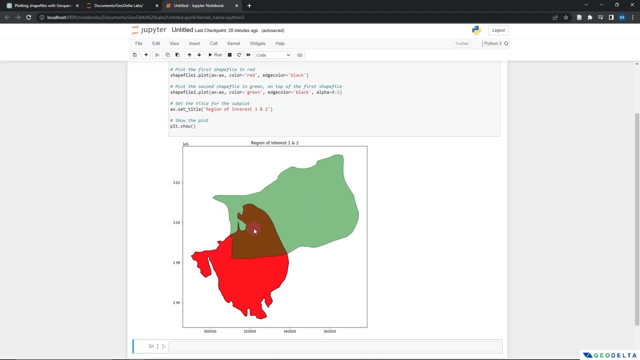 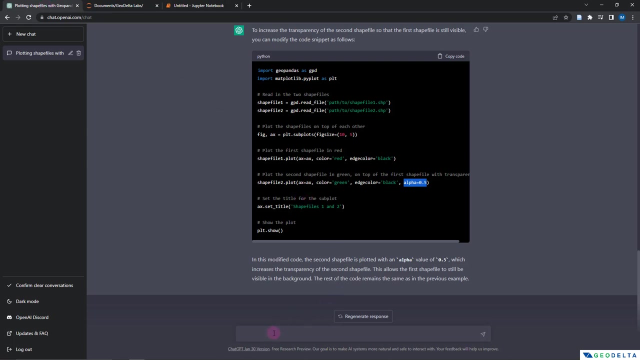 two different shapefiles and get the extent of the polygon that basically common to region of interest one as well as region of interest two, and calculate the area of that and export that as a CSV file. So what I'm going to do is I'm going to head back to chat GPT And over here. 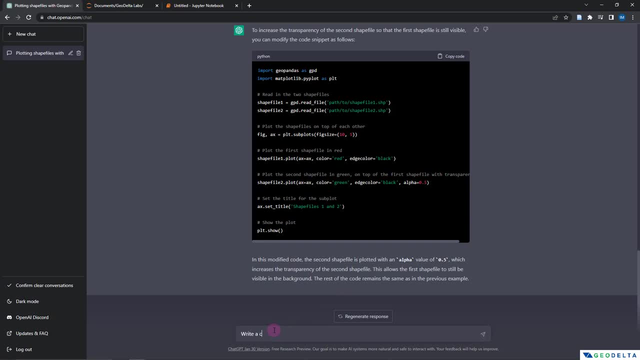 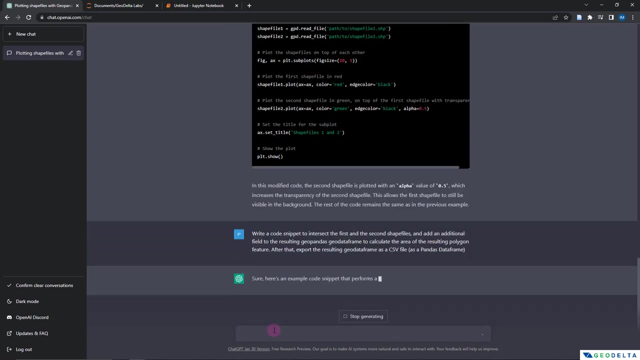 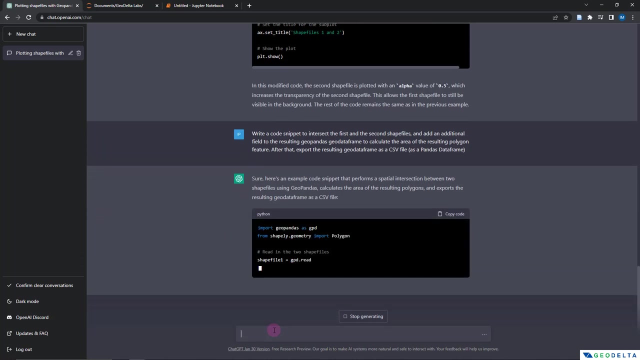 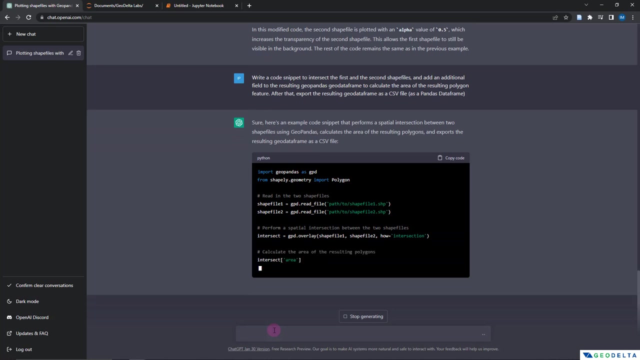 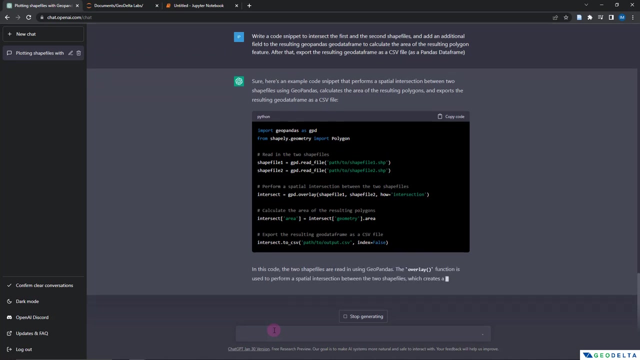 I'm just going to basically slide in my request again. All right, let's hit enter and see what sort of a response we're going to get from chat GPT. All right, now let's go line by line and see what it's doing. So over here you can see that it's. 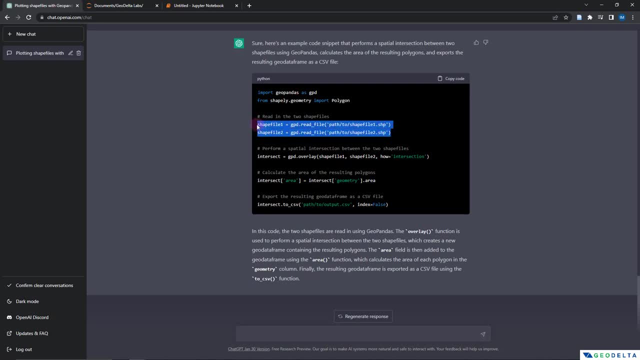 basically asking us to import the two shapefiles again, which we already covered in the first exercise, And now it's running basically an overlay operation. But, if you were to be specific, it's basically an intersection operation Between the first shape file and the second shape file And it's basically making use of the Geo. 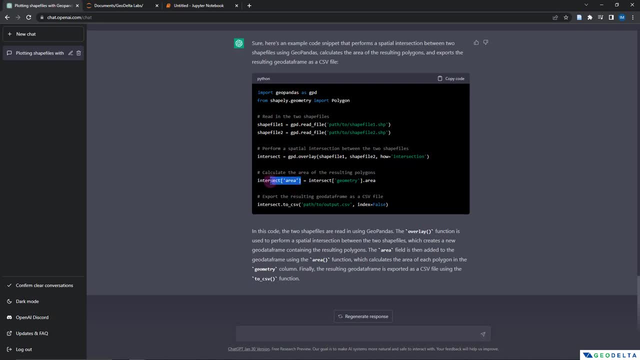 pandas library to do that, And after that it's basically including a new field called area or a new column. If you were to actually refer to the attributes table as a table, it's basically adding a new column or a new field called area, And this is how it's basically calculating the area. So so, 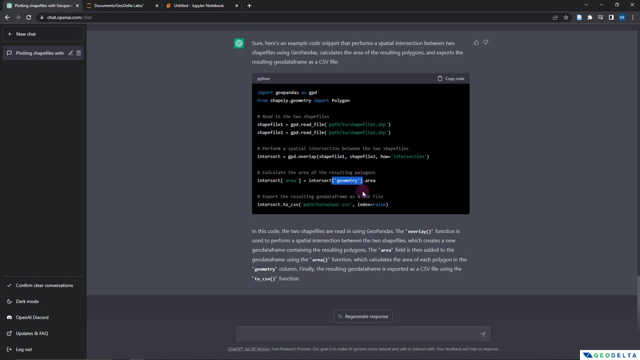 here it's referring to the geometry column which we will also see as we go along. what this geometry column refers to. in case if you're not really familiar with why we have a geometry column in this intersect Geo pandas, Geo data frame, And what this dot area does is it's basically calculating the area And finally it's 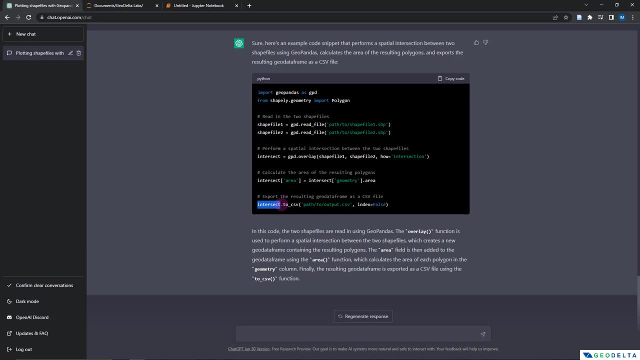 exporting this intersect Geo pandas Geo data frame to a CSV, And when you do this it's basically losing all of its geospatial properties, And over here we can specify the path to which we would like to export this file. All right, if that was too much information, let's dissect this part by. 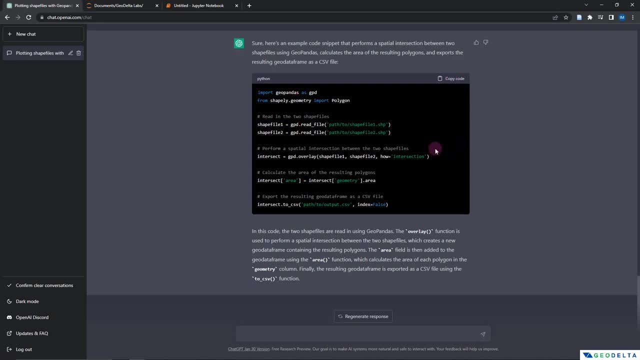 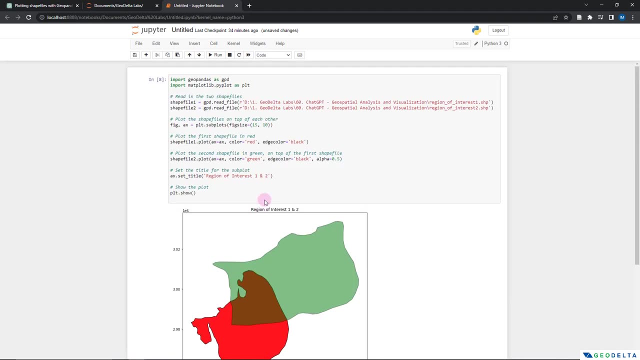 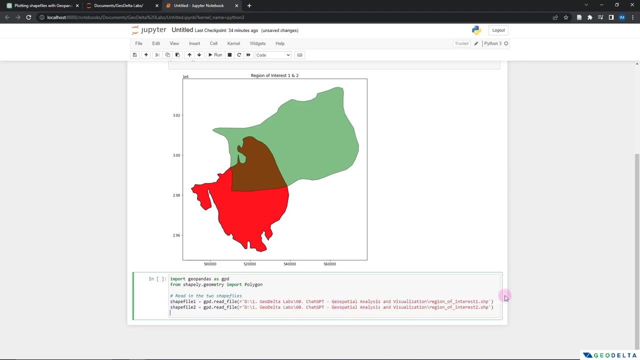 default. So what I'm going to do is I'm going to basically use these two blocks And I'm going to use a new line over here And, sure enough, we are going to replace these two lines by the actual path. And now, if I run the code, you can see that we didn't really get any error messages, or 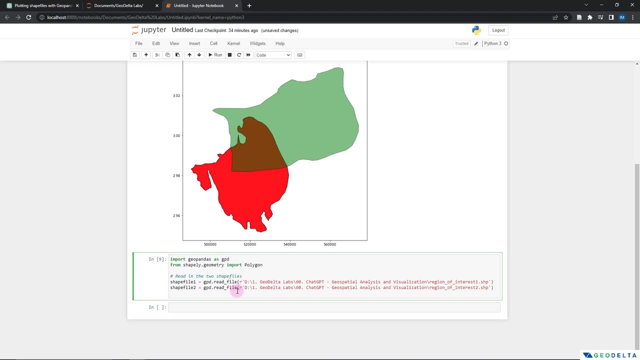 anything. And now, for the first time, we are going to actually explore the attributes table of the two different shapefiles. So if I would like to view all of them, I'm going to do that And I'm going to call this shapefile One looks. what I can do is I can maybe move to another line and 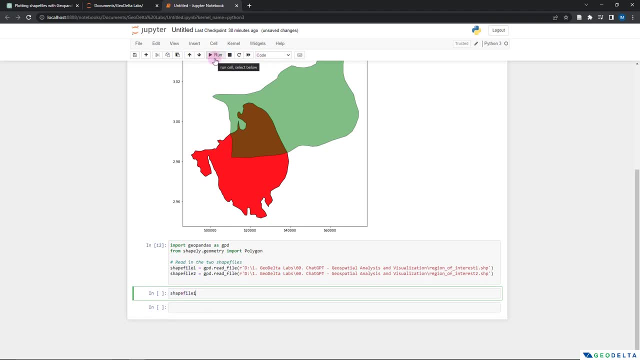 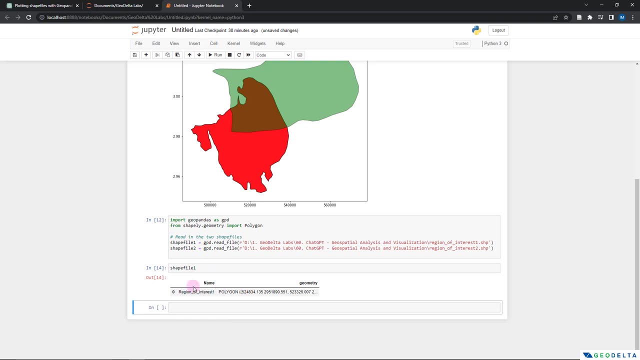 type: shapefile one. So let's go ahead and run this cell And this is how the attributes table of the shapefile one is supposed to look. To be frank, we no longer call this an attributes table Once we import this into Python using Geo pandas. we need to start calling them Geo pandas, Geo data. 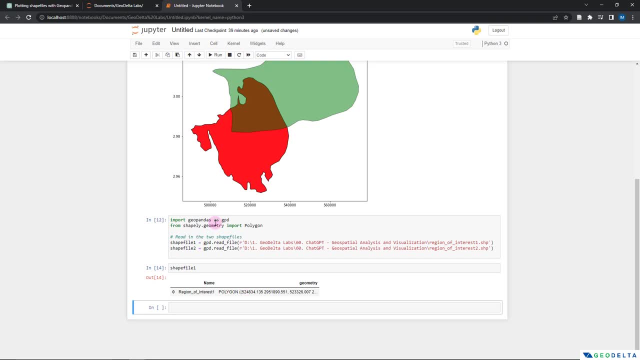 frames. Well, if you were to be pedantic, but yeah, that's the correct term that we're supposed to use. So when we look at this table, we're going to call this table. we're going to call this table this Geo pandas, Geo data frame. you can see that we have two different columns, So the first one is: 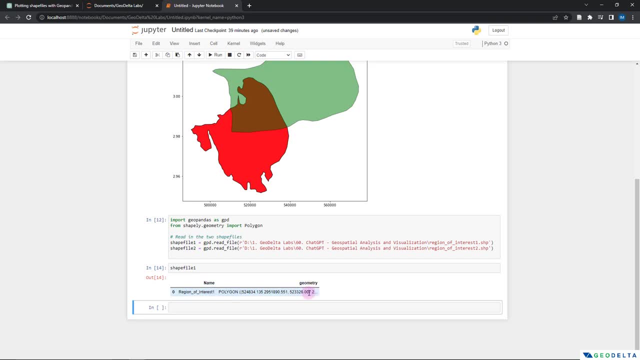 called name, And there's this geometric column which basically gets created every time when we import shapefiles into Python as a Geo pandas, Geo data frame. It's basically a special column that embeds the geometrical properties. Without this column, we wouldn't really be able to plot. 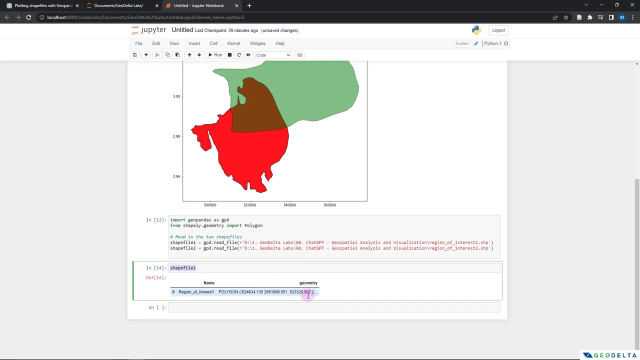 this shapefile one, because this column is the place where the geospatial properties are basically saved. It wouldn't really know how to draw it. So we're going to call this column And we're going to draw a polygon object if it didn't really have this geometry column. So that's a bit of extra. 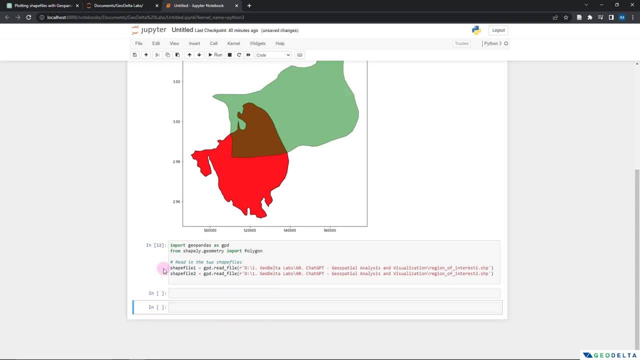 information. So let's get rid of this and head back to chat GPT. And now I'm going to copy this line of code and edit over here And instead of the name intersect, I'm just going to modify it slightly by saying intersected object, just like that, so that it would be clear we are not referring. 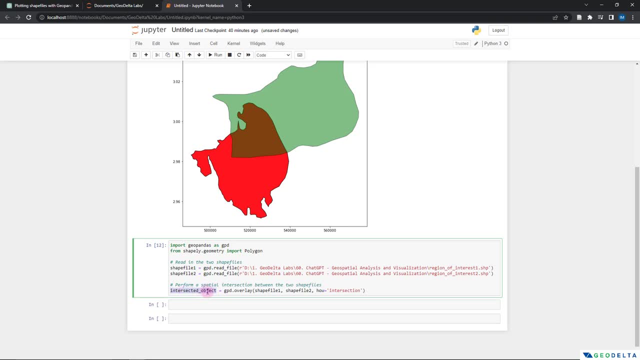 to the process of intersecting. We are referring to the object, we're just passing a name over here And if you run this command and if I want to inspect this intersected object, if I run this cell now, you can see that this. 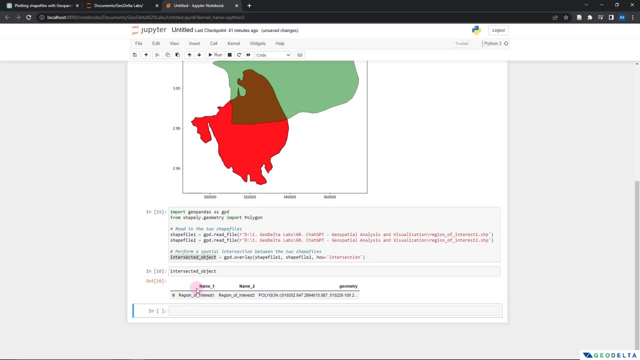 intersected object basically has properties from both name one and name two, And if I want to visually see how this intersected object basically looks, what I can do is I can- Well, I can ask that from chat GPT as well, But it's not that significant. All I have to do is 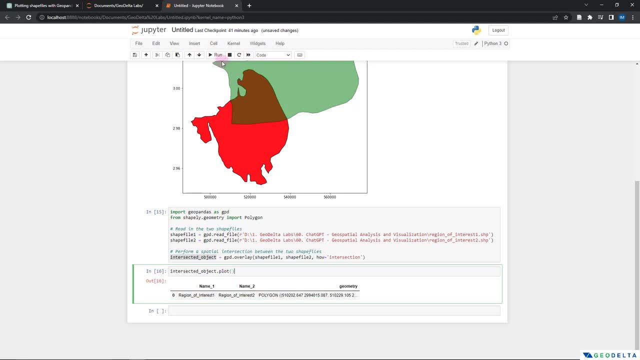 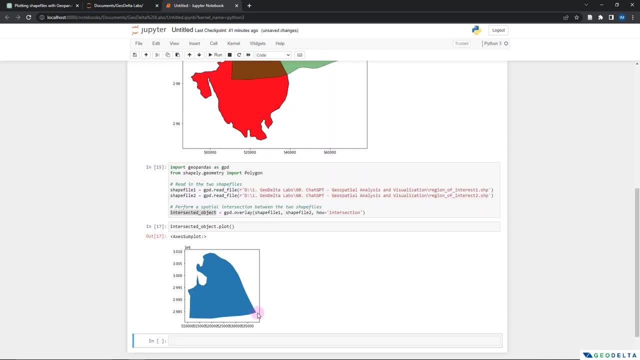 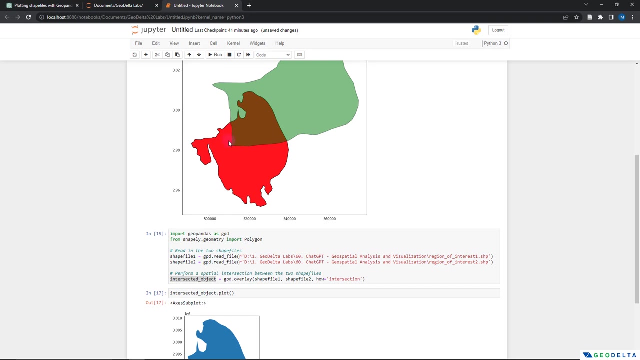 just pass a dot plot over here And if I run this cell, it's going to basically create a plot which corresponds to this intersected part. you can see that the southern boundary is basically the boundary right over here And this part in the west is basically the boundary over here And the 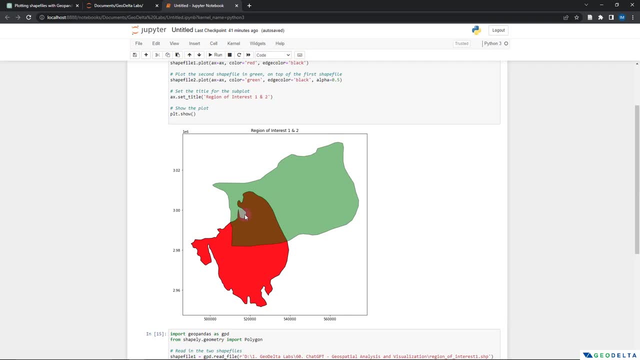 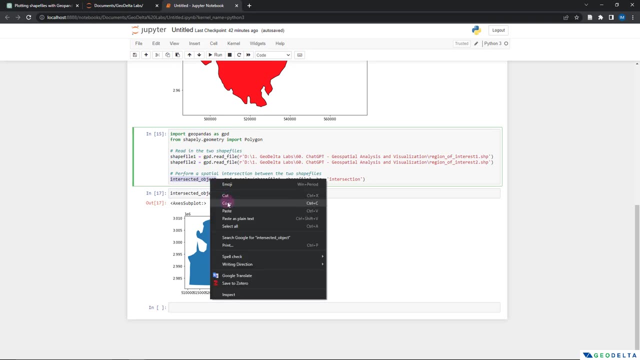 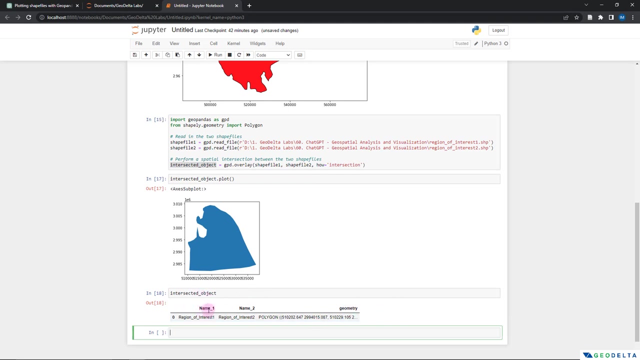 remaining part has been taken from the extent of basically the shapefile one, as we can see right over here. And just so that we don't forget, let's copy this And see how the attributes table or the Geo pandas geodata frame looks. So you can see that currently, 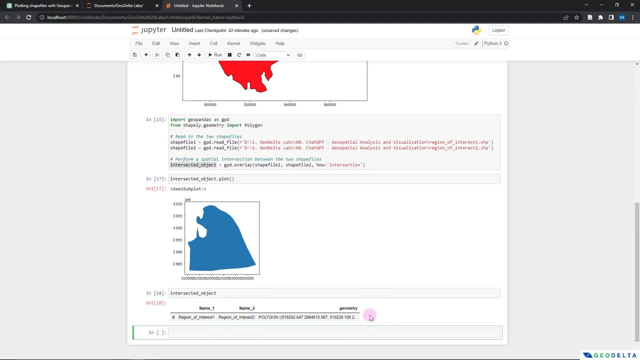 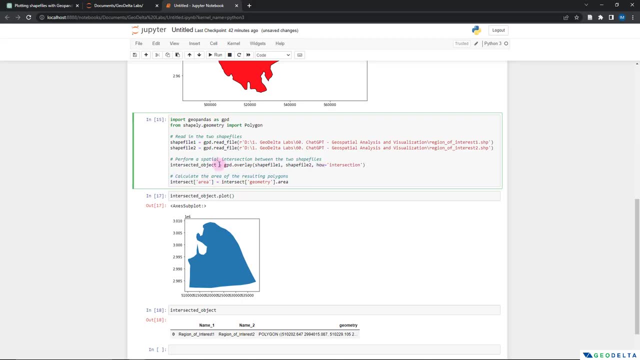 we have three different columns, name one, name two, And in this line what we're trying to do is we're basically trying to create a new column called area. So we here we will need to change the name as well to intersected object, And the same goes to here as well. And now, if I select this cell and 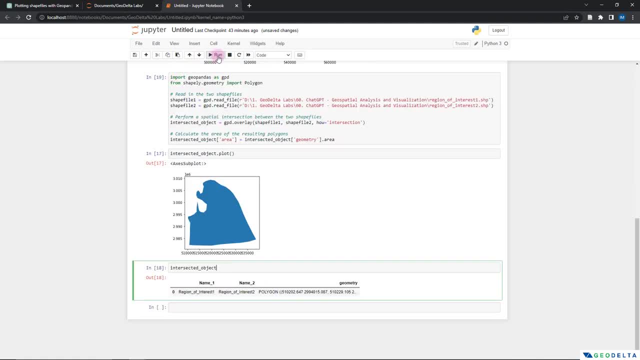 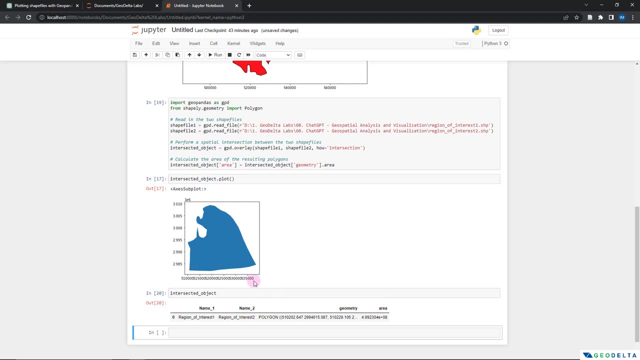 run and if I go over here to this cell and run it as well, now you can see that it's basically having a new column called area. Now, since by default it's using meters as its units, we are getting this area in. 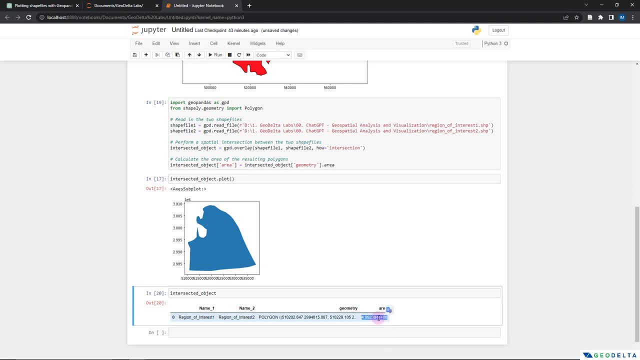 square meters, basically, But if you wanted to, let's say, convert it into square kilometers, because the numbers look too big over here, you can see that it's basically going to 10 to the power eight. what we can do is we can simply divide this by 10 to the power six. 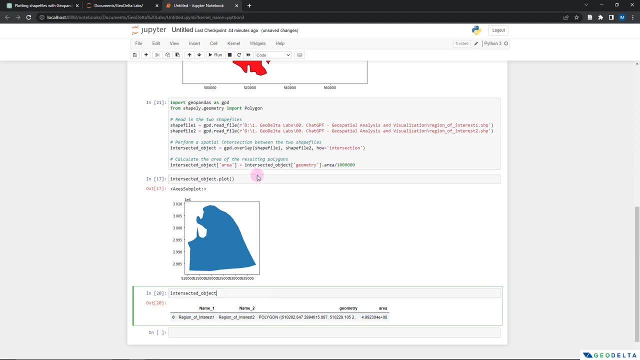 And rerun the cell and select here and rerun this cell as well. So we're here. you can see that it's perfectly coming up to be about 499 Square kilometers the extent of this intersected object. And finally, how do we export this? we can add another line of code and specify the. 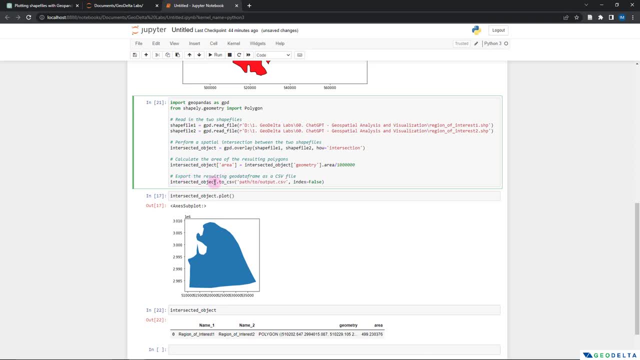 name of the shape file over here or name of the gym and thisEO Calendar frame, over here to be intersected object to CSV and over here we can set the path as well and the name of the CSV file. I can name it as intersected object dot CSV and we'll see what happens if you run. 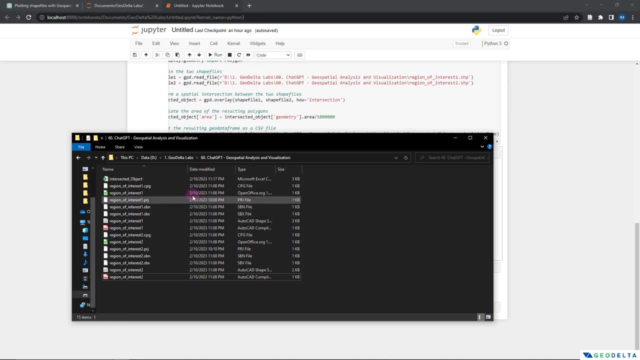 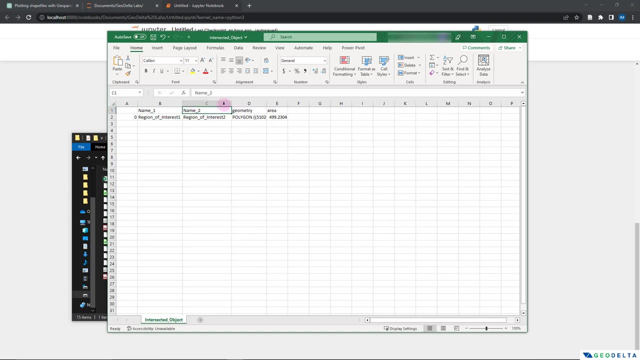 the code. so, sure enough, you can see, over here there's one CSV file called intersect object, intersected object- and if I right click and open that up, this is how it's going to look. so we have, well, these columns, name one, name two, which indicates that the area, the common area, has parts from both region of 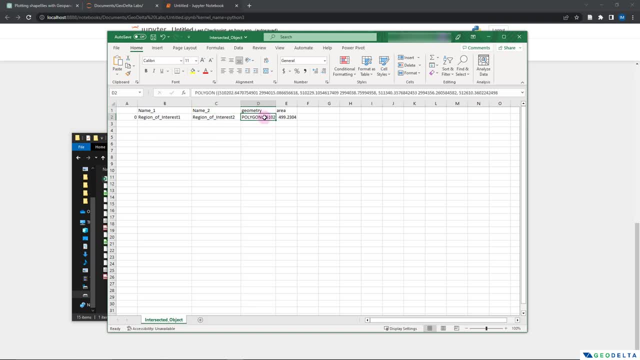 interest one and region of interest two, and the geometry column wouldn't really be necessary for us, so we can just right click and delete and we have the area over here. now you can see that it's just one line or one row, but if you're doing 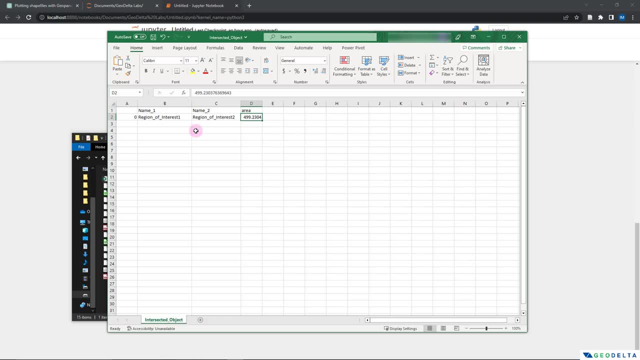 this using complex shapefiles, which has maybe thousands of different objects. the parts that get intersected will be completely different and the numbers will be way higher than this, so in such a case it would be quite handy to have them exported into a separate CSV file, like this, but just for the demonstration. 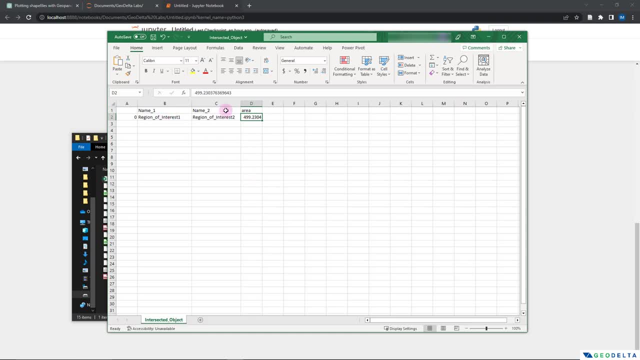 purposes of this tutorial, basically using a very simple example which has just one row. however, the principle of doing things, or the order of doing things, remains to be the same, so that you can extrapolate the skills that you're learning from here into your own different specific cases and see how it. 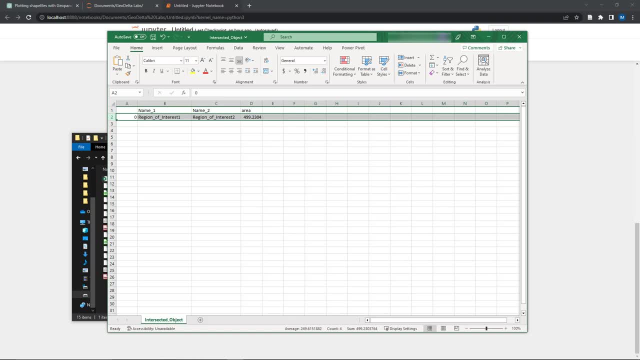 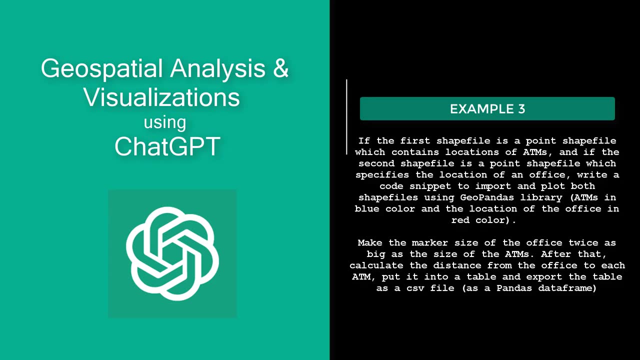 goes from there. alright, guys, so that's about it for the example number two. now let's move on to the example number three. alright, so example three goes like this: if the first shape file is a point shapefile which contains locations of ATMs, and if the second 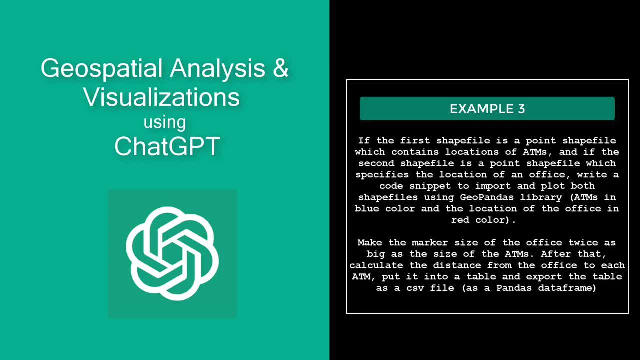 shapefile is a point shapefile which specifies the location of an office. write a code snippet to import and plot both shapefiles using geopandas library and I'm specifying that I would like to have the ATMs in blue color and the the office in red color And I'm also specifying that the marker size of the office is required to 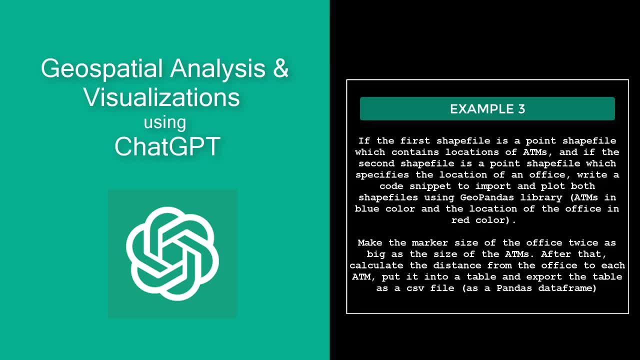 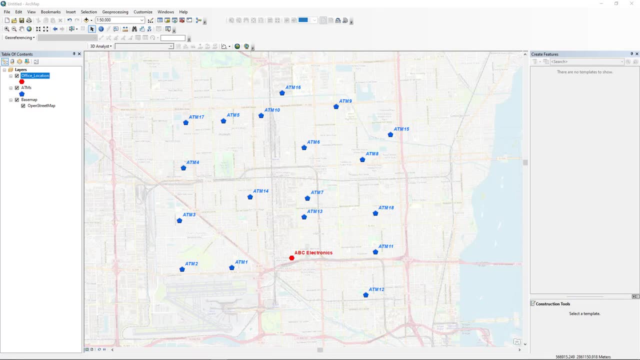 be twice as big as the size of the ATMs, And after that I would like to calculate the distance from the office to each ATM And I would like to put it into a table and export that table as a CSV file or as a pandas data frame. Now you can see that the complexity of the problem compared to the 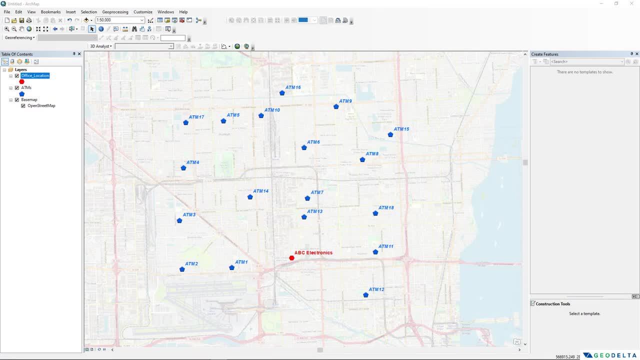 previous case might be a bit high, because when we specify the problem, you can see that we're actually being more specific when it comes to what we need to do, And now we're dealing with points instead of polygons as compared to the previous two examples. And before we proceed with generating, 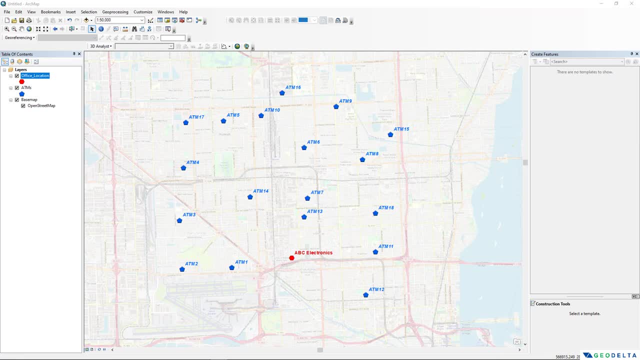 the code snippet using chat GPT. I would again like to give you some sort of an overview of how spatially these points are supposed to be. And again, I'm using ArcMap just for the demonstration purposes. you don't really have to worry about this part at all. 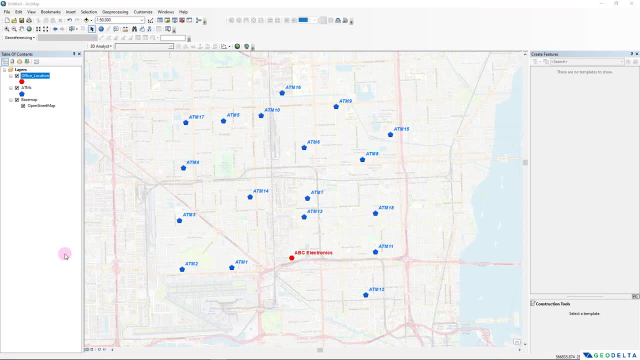 Except for understanding what sort of what sort of a data set that we're actually dealing with. So, as you can see, over here I have, I guess, about 18 different ATMs which are marked just like this, in blue color, And I do have one office location called ABC Electronics, which is marked in red. 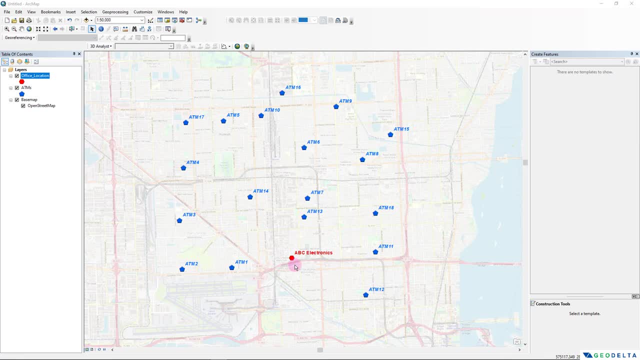 color right over here. So the objective of this exercise would be to generate a code that can calculate the distances between, let's say, ABC Electronics and ATM one, ABC Electronics and ATM two, ABC Electronics and ATM three, and so on. Well, if you were to do a manual calculation, 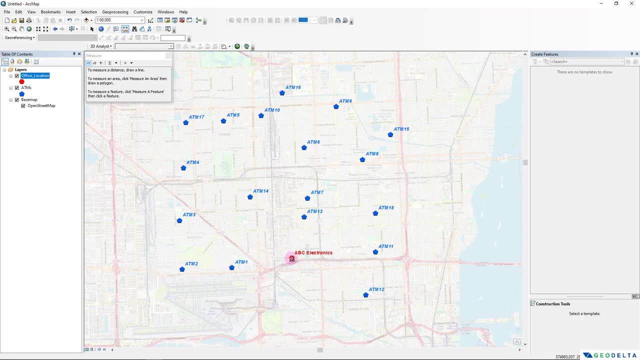 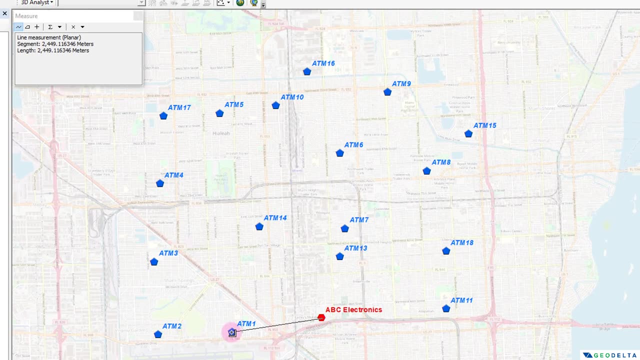 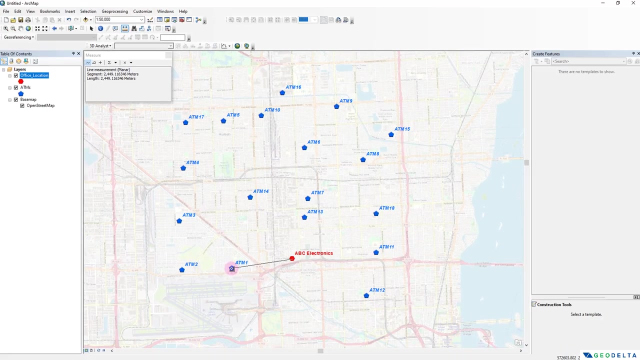 using a software like this, let's say, for the distance between ABC Electronics and the ATM number one, we're supposed to get a distance of about 2.5 kilometers. Well, I'm not being very precise over here. However, when we use GeoPandas to actually calculate these, 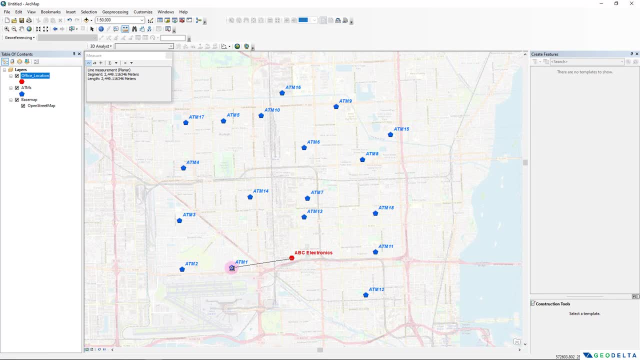 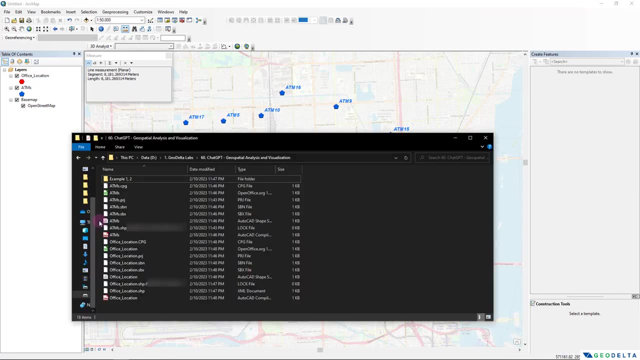 distances. we're going to get exactly the precise values when it comes to the distances between ATM ATMs- ATM two to ATM three, ATMs four, ATMs five and so on- And if you try to see visually how these shapefiles look. so here you can see these files that basically make up the ATM shapefile. 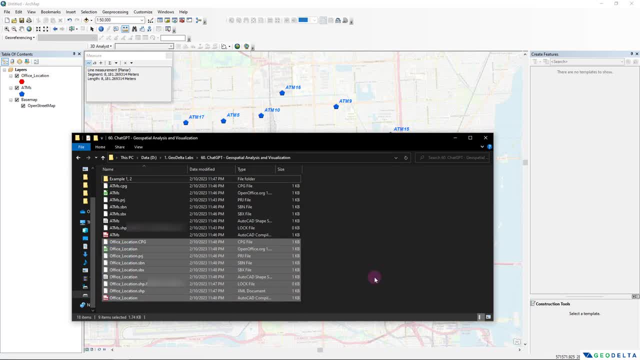 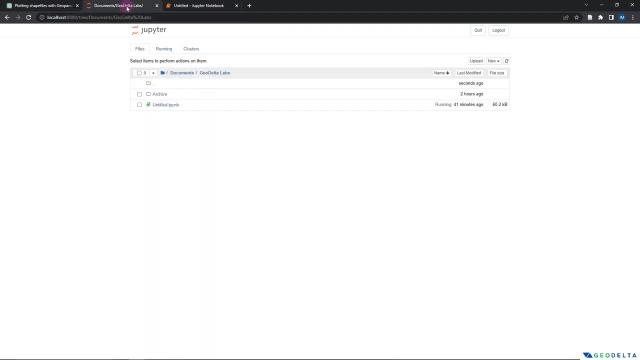 And similarly, we have the files that basically make up the office locations as well, And since this example is basically not related to the example one and example two, what I'm going to do is I'm going to name this as example. one is actually not related to the graphic name. I'm going to name THIS one as example. 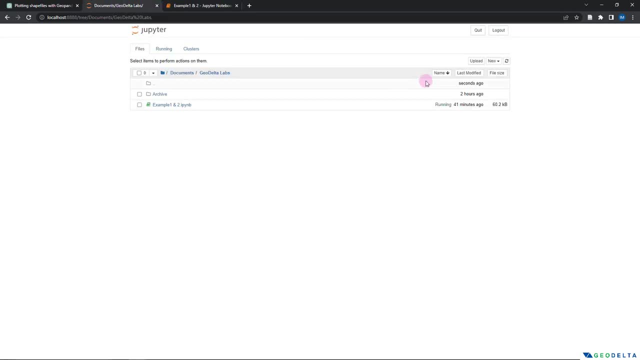 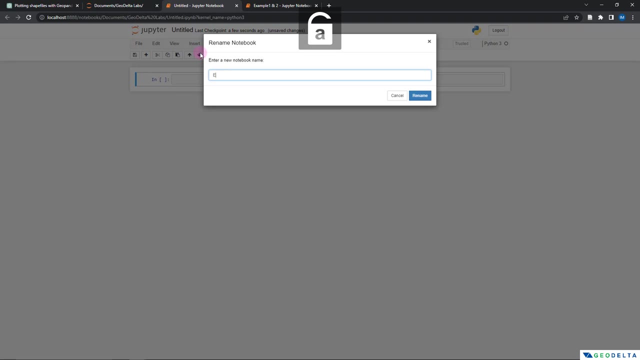 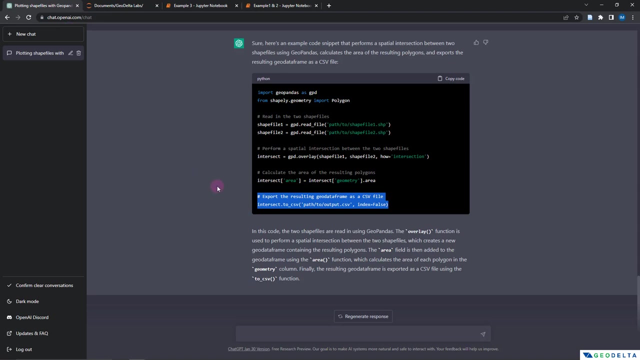 one and two, And I'm going to create a new notebook, And for now let's call this example three, And what we can do is we can basically head back to chat GPT as well. And again, since what we're trying to do is not really related to the 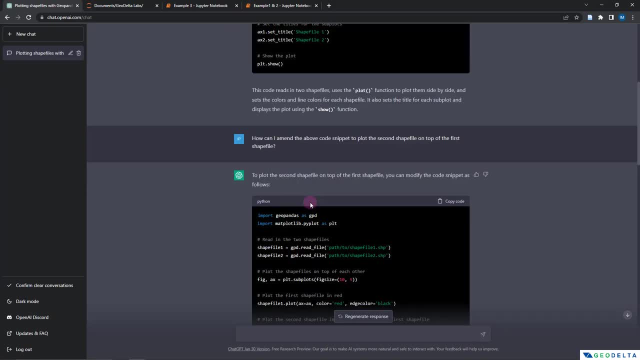 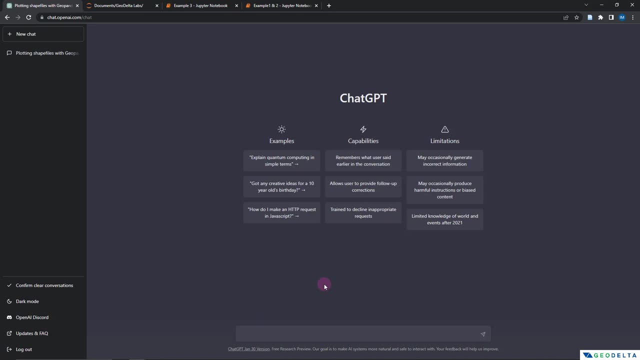 conversation that we were having with the chat GPT. Until now, what we can do is we can actually open up a new chat And simply specify our request. Alright, so that's going to be our request. After that, we can simply hit enter to see what sort of a response we are going. 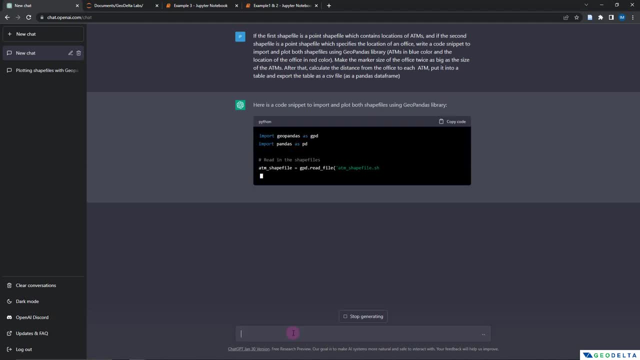 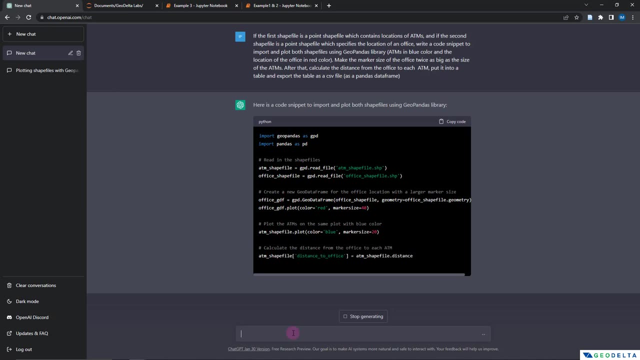 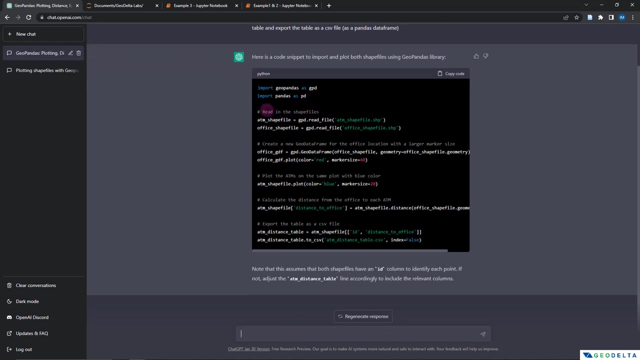 to get from chat GPT And, as you can see, it's basically writing out the code for us. it's using pandas this time, in addition to the Geo pandas library, And, first of all, what it's doing is it's basically using 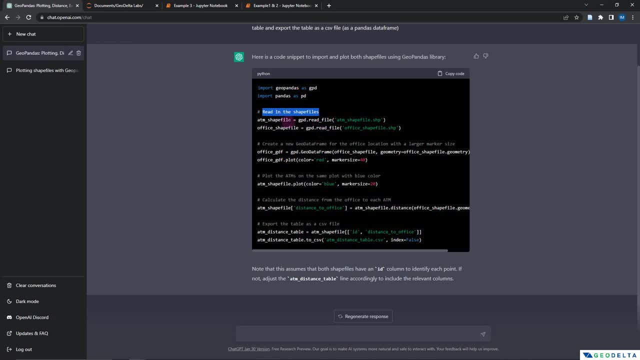 its reading in the two different shapefiles. So, even though the shapefile, the name of the shapefile that we specified in our own case was ATMs, you can see that it's again assigning a very descriptive name for the shapefile, so that we will know. 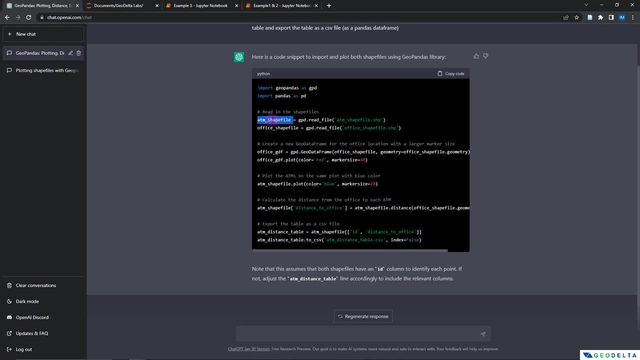 exactly what which shape file it's referring to. So it's creating a shapefile called ATM underscore shapefile and followed by another shapefile called office underscore shapefile. And when you import this shapefiles into Python using Joe pandas library becomes Joe pandas- Joe dataframes. So it's somehow adding this extra. 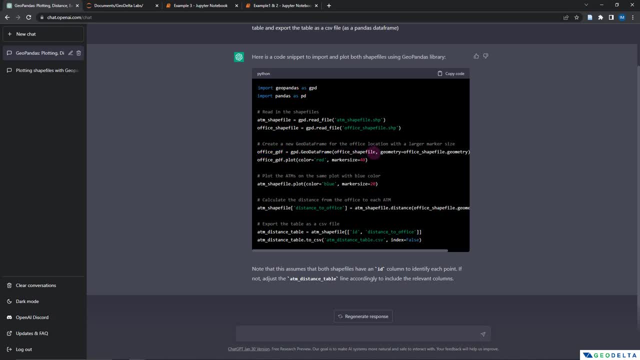 line of code to basically convert this office shapefile into a Joe pandas Joe dataframe for the second time, which I don't think is actually going to be necessary to be able to do this, However, they're just sliding this code in And what's going to be? 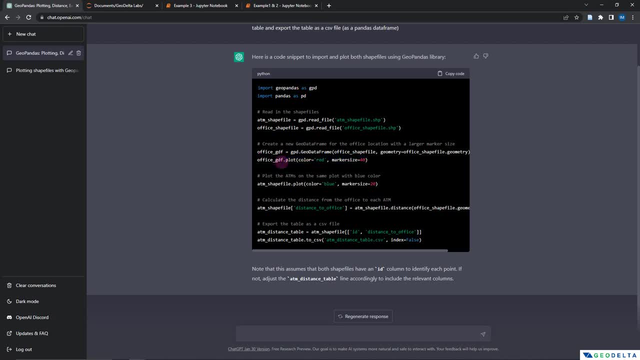 important for us is that it actually understood that we wanted the marker size of this office GDF to be twice as big as the marker size of this ATM shapefile. So over here you can see that as an example. it assigned 20 as the marker size. 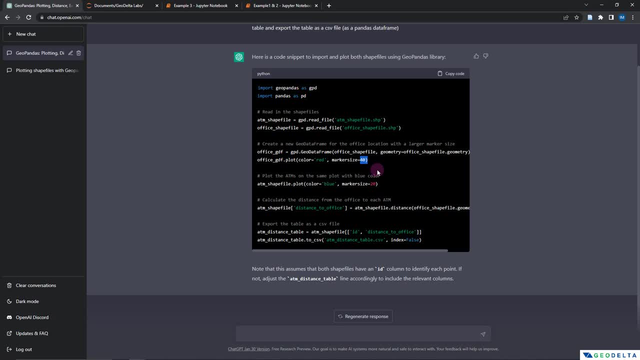 and this one is double of 20.. So it actually understood our command, along with the requests when it comes to how I would like them to be colored. This one is will be in red and this one will be in blue, And after that it's basically doing the computation of the. 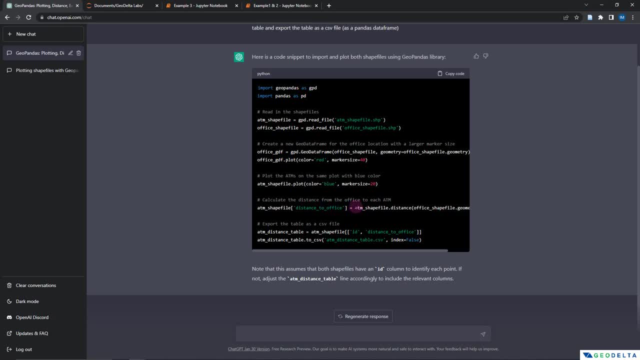 distance between the location of the office and each of the different shapefiles. And over here, what it's doing is basically adding a new column or a new field called distance to office to this ATM shapefile, And it's calculating the distance between each of those different ATM points. with respect to this, 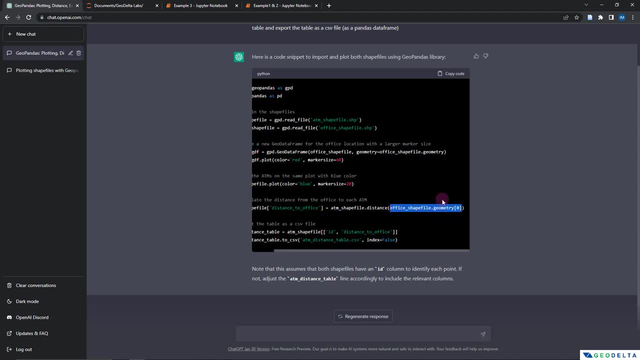 geometry column of this office shapefile. So we'll actually get into this in a bit of a detailed way, when we when we're actually executing this code And finally it's exporting that, that data table into a CSV file. So here it's basically assuming that. 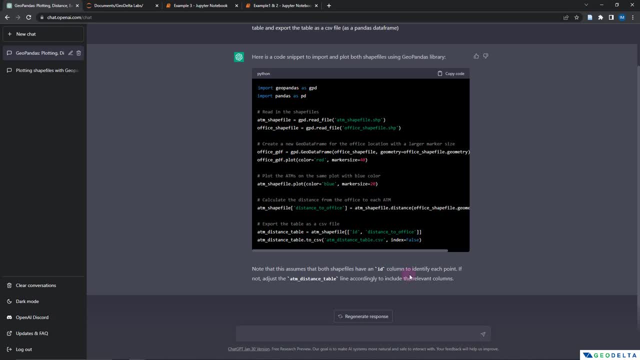 both the shapefiles will have an ID column to identify each point, which might not necessarily be the case, but it's always good to have this kind of a footnote so that we know exactly what we have to deal with. And it's asking us to basically adjust. 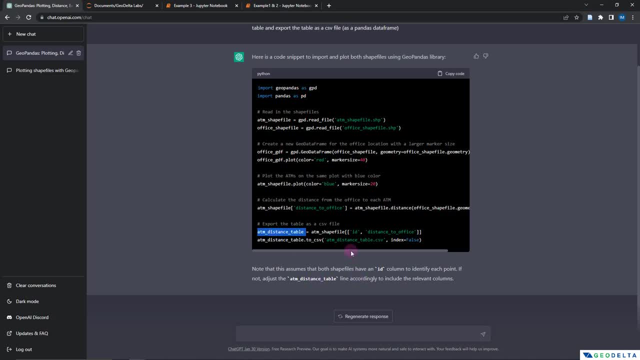 this ATM distance table if we happen to run into issues due to not having this ID column. So we'll get to that once we reach that point as well. So, as a starting point, what I'm going to do is I'm going to copy this: 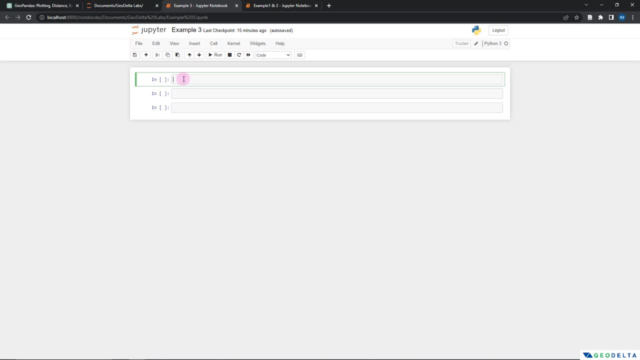 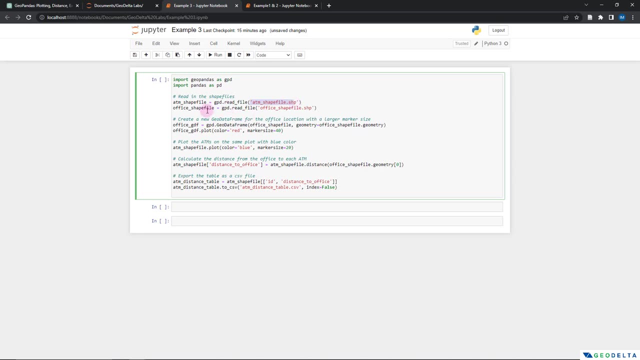 code and paste it right over here, And, sure enough, we are going to have to change the paths to this ATM shapefile and the office shapefile as well. So the first one was called ATMs- dot SHP, And similarly, the second shapefile was called 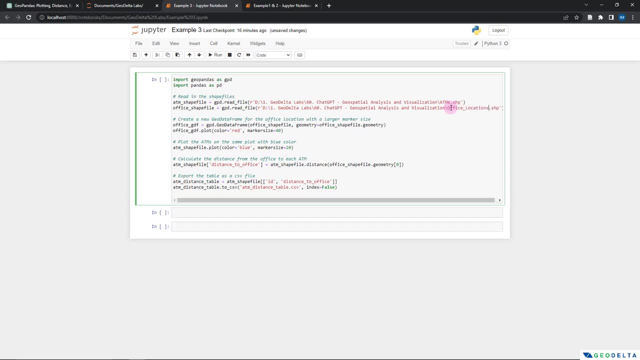 office locations, SHP, And. and I think we don't really need to change anything in these two lines of code, because it's basically assigning the color and the marker size And again, for some reason, it's basically writing this again into a new. 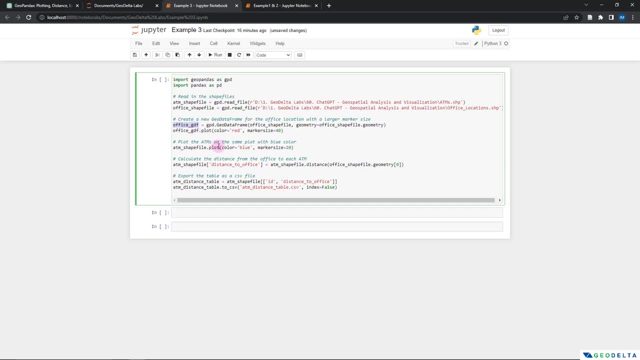 geo data frame, called office underscore GDF, which I don't think is actually an absolute must. However, we'll just go along with that. So what I'm going to do is, before we explore these two lines of code, I'm just going to come in these two lines out and this line as: 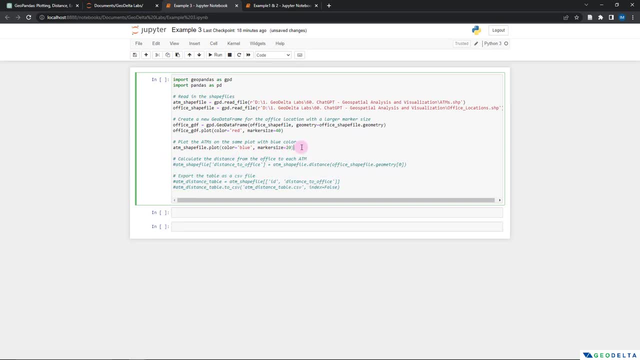 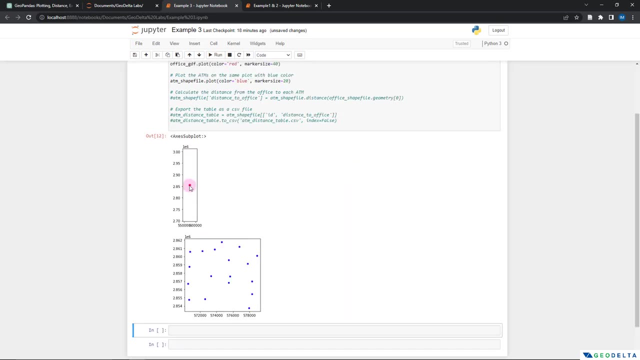 well, so that this won't be sort of executed when I run the code snippet. So let's run this one and see, And over here you can see. the first plot is basically showing the location of the office and the second plot the locations of the ATMs. Well, 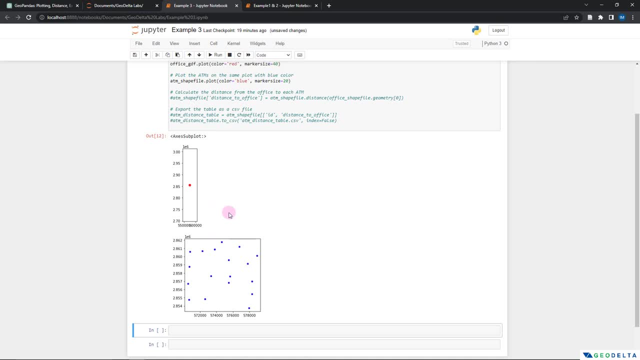 just because I was not really specific when it comes to asking chat GPT to provide the code to plot both of these shapefiles on the same plot. It just plotted these two as two different plots. However, that's totally fine in case if you want to amend the 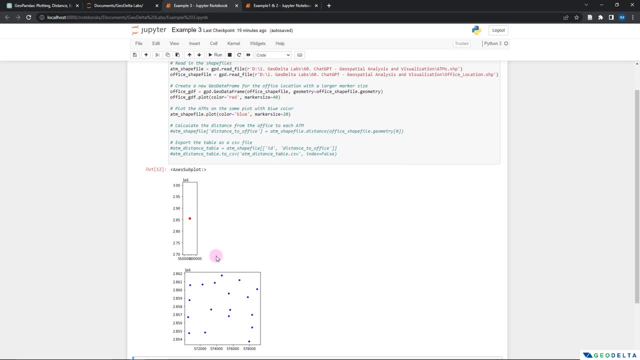 code to plot both of these shapefiles on the same plot. You know how to do that, especially if you were to refer back to this code snippet of example one, And you will be able to amend the code accordingly. However, for this example we have a. 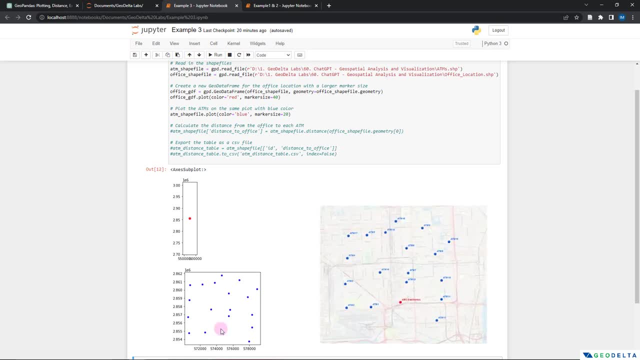 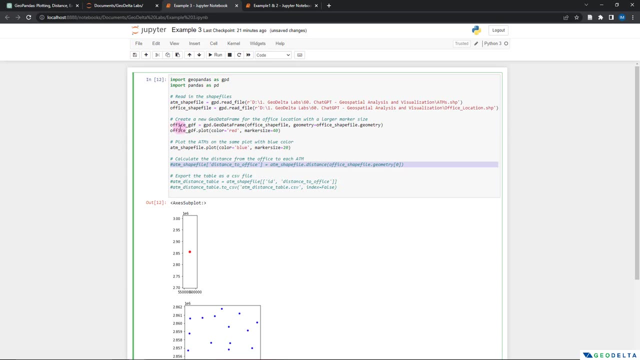 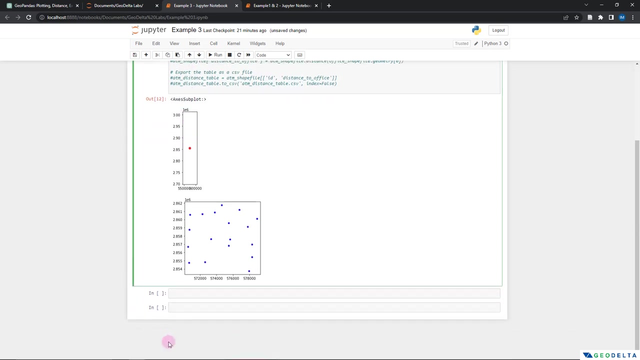 proper understanding of where this office location point is actually supposed to be. And before we go ahead and activate this line of code, let's see how the attributes table of each of these different shapefiles actually look. So if I open up the office GDF, so this is how it looks- you can. 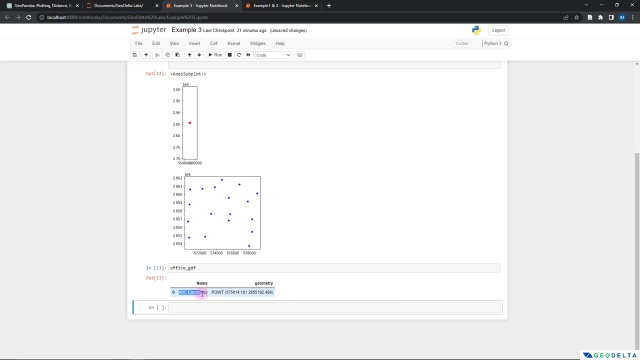 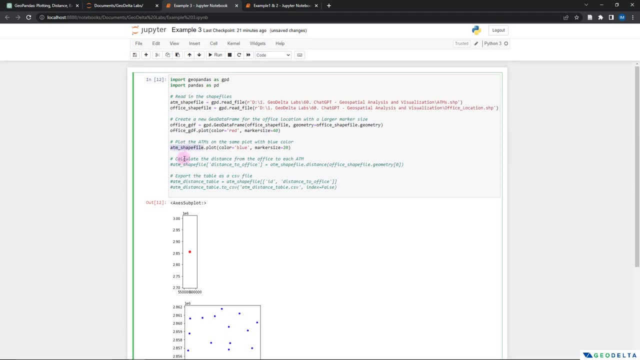 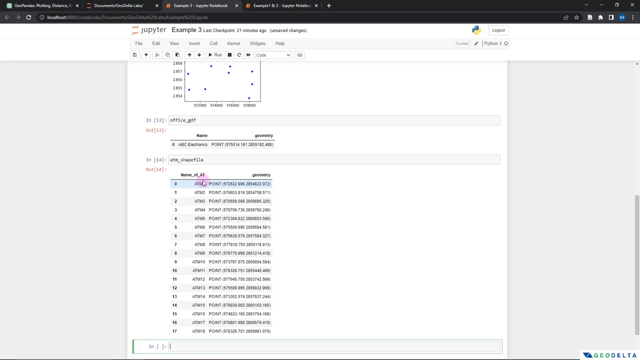 see that there's one column called name and the name is ABC electronics And we have this special geometry column as well. And similarly, if I were to explore this ATM shapefile, GeoPanda's GeoDataFrame, you can see that there's one column. 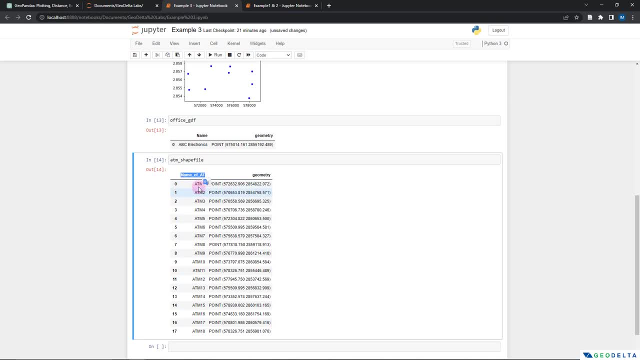 called name of AT. Well, actually it's supposed to be name of the ATM, And over here you can see that each ATM has its unique name, starting from ATM one to all the way until ATM 18.. So each of these different points do have its unique ATM ID. 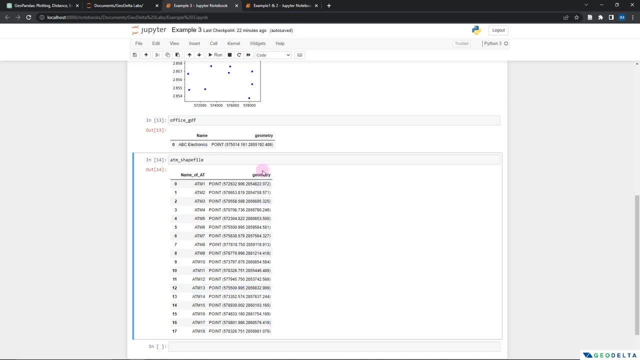 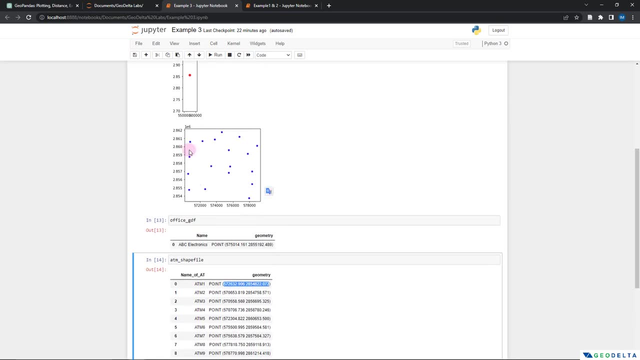 name as well, Obviously in addition to this special geometry column which specifies the x and y coordinates so that it knows spatially where it's supposed to be when we talk about a geospatial plot like this. All right, now what I'm 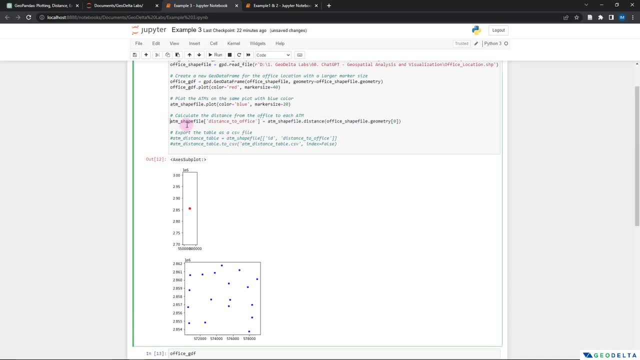 going to do is I'm going to activate this line of code, And what this does is it's going to basically add a new column, heading called distance to office, to this ATM shapefile. So right now you can see that we have just two columns, name of 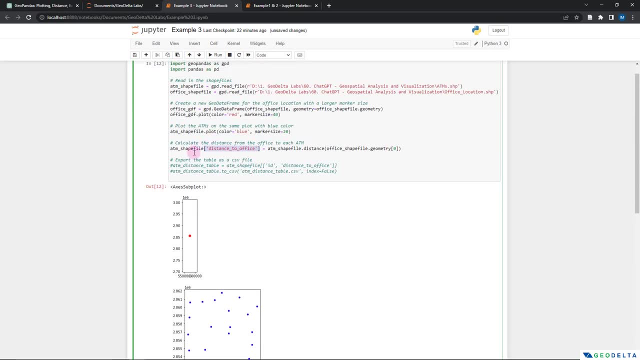 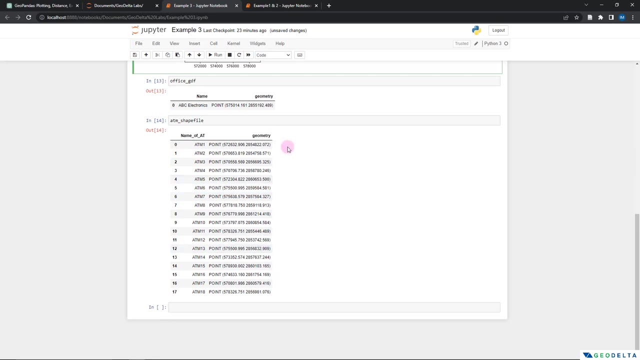 ATM and the geometry. So once we execute or once we run this line of command, what it's going to do is it's basically going to add a new field called distance to office, maybe somewhere over here, and it's taking the ATM shapefile And it's calculating. 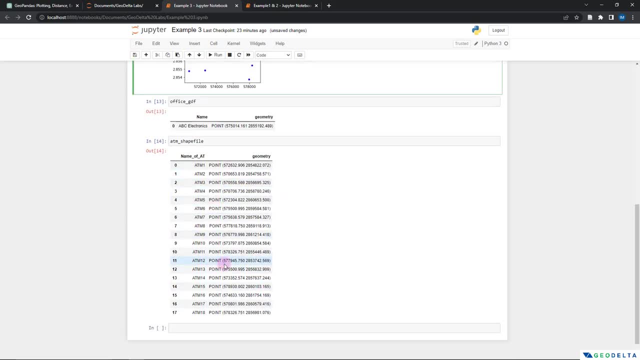 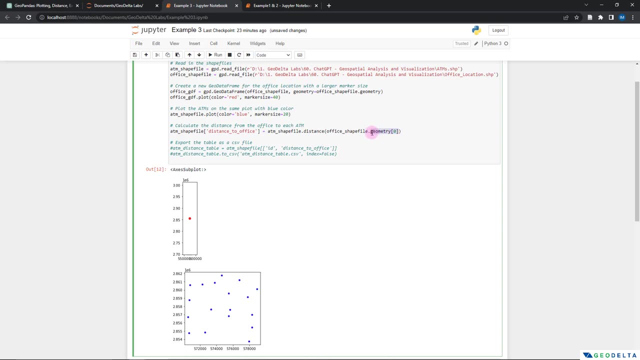 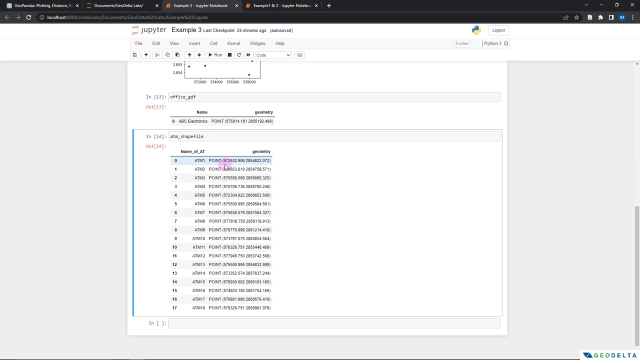 the distance from each of these different 18 points to the spatial location of this office shapefile, which is specified by this geometry column right over here. So when we say a distance calculation, what we're actually referring to is basically the distance, the spatial distance. 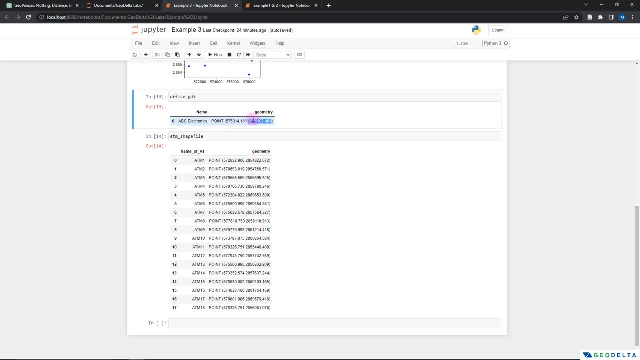 between this x y coordinate and this x? y coordinate And that's going to give us the distance between ATM one and ABC electronics. And, similarly, if I were to calculate the spatial distance between this point, which is given by this x y coordinate, 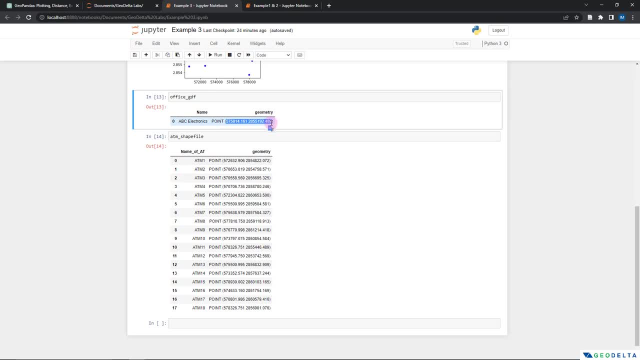 and this point, which is given by this x- y coordinates, that's going to give me the distance between ATM two and ABC electronics And, similarly, what it's going to do is it's going to perform that operation for all the different 18 points And 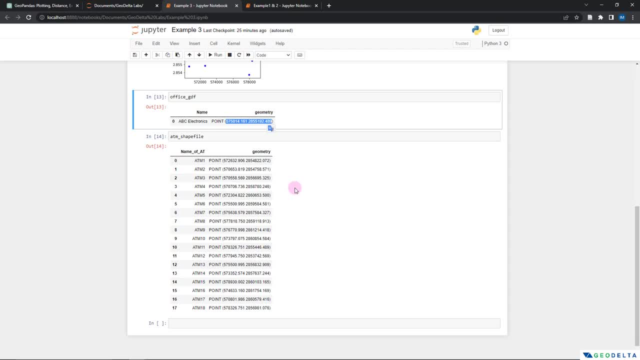 it's going to create a new column on the right side and probably stack it over there saying this is the distance between the ATMs and the office location, which is ABC electronics in this case. Alright, so let's run this code snippet: 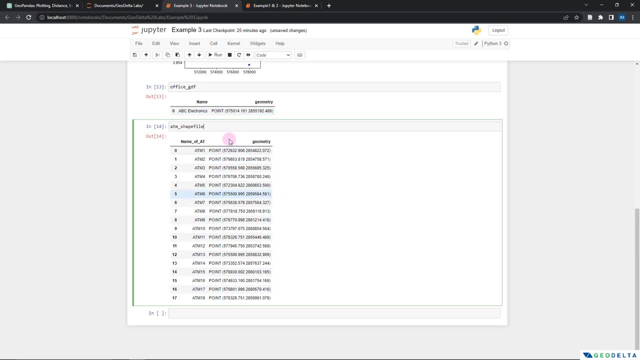 And after that we would have to run this one as well. And sure enough, you can see a new column appears right over here, which is basically the distance calculation between all the ATMs and the location of ABC electronics. If you guys can, 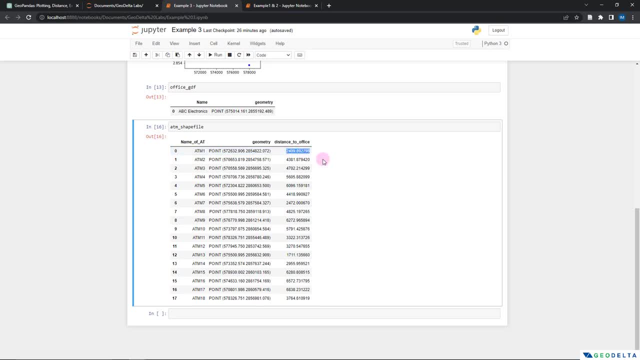 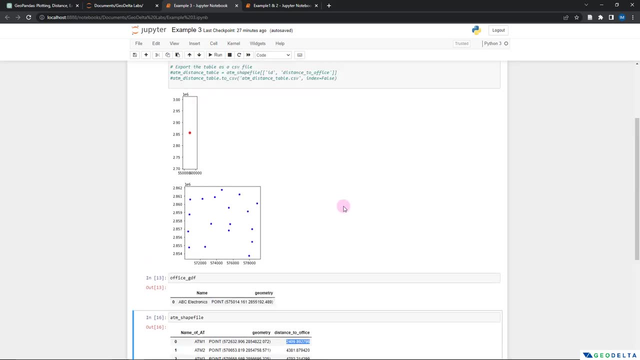 recall when I calculated the distance using ArcMap just to demonstrate to you guys, at the beginning of example three, I can recall I got something which is close to this number. And finally, let's head over to this and see what we have to do when it comes to exporting this tabel. 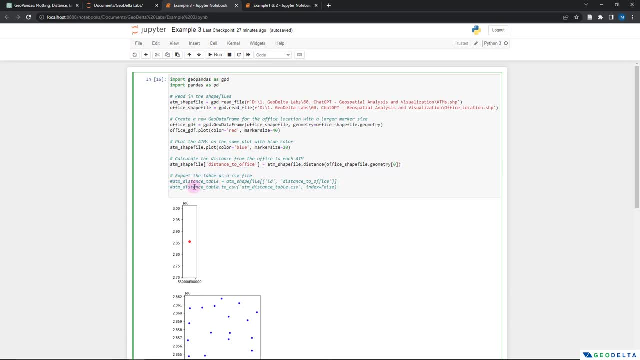 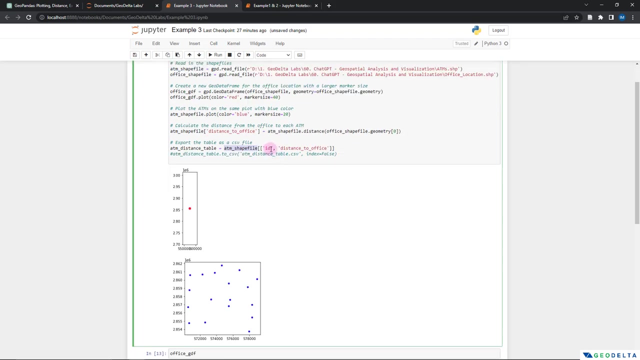 as a CSV file. So if I acti this first line of code, yo can see what it's going to do. is h basically creating a new variable called atm underscore- distan s underscore table, and it's taking this ATM, Geo, pandas, Geo DataFrame And it's basically stripping off all the unnecessary. 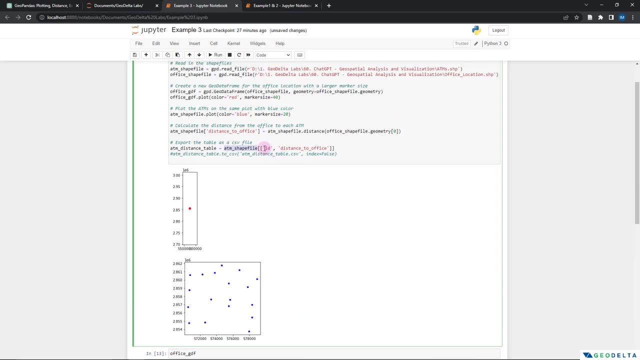 columns, Let's si if you've had multiple columns, what it's doDel ing over here is basically manu 어 strainsgeben çocuğ of columns, or just the column IDs that we would like to have in our final exported product. 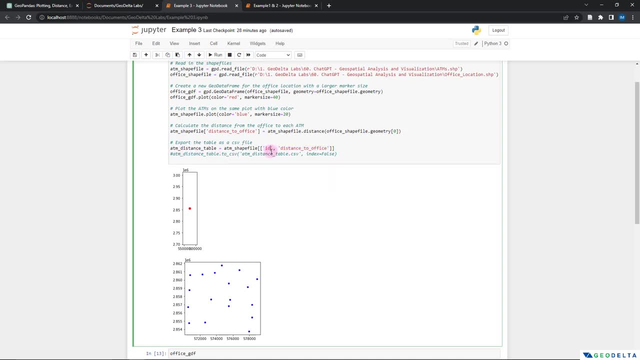 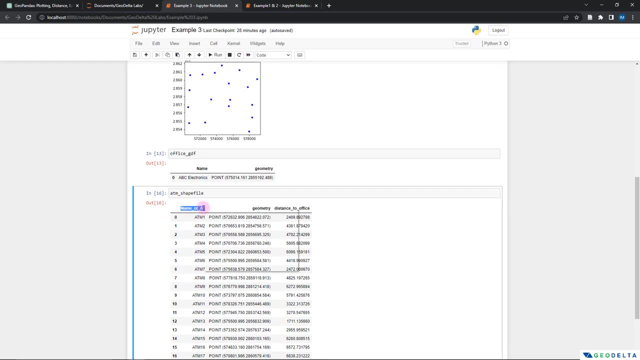 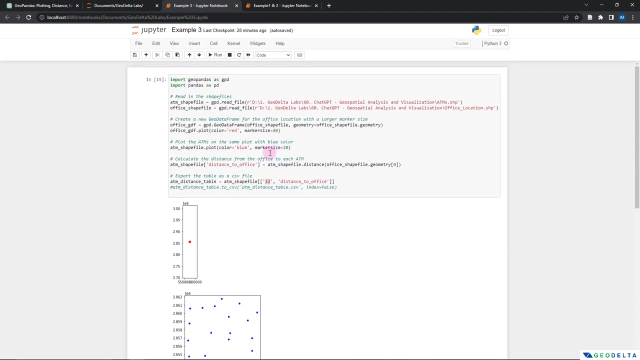 which is going to be this ATM distance table, And since we do not really have a column called ID, what I'm going to do is I'm going to copy this name because in the final output, I would like to have this column which specifies the ATM ID as well. So I'm just going to replace this with that. 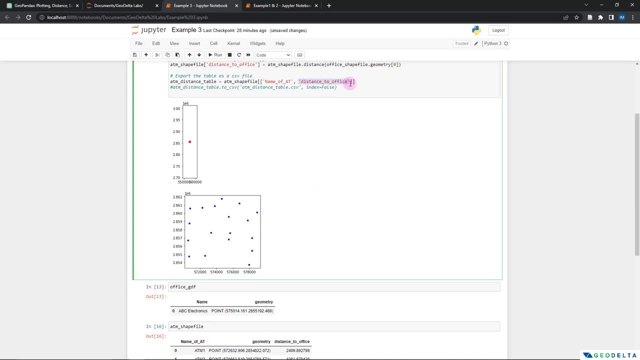 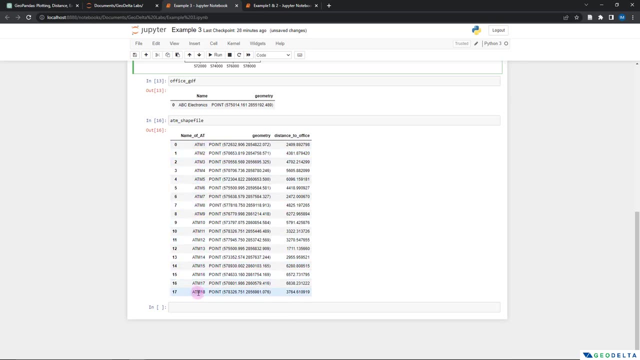 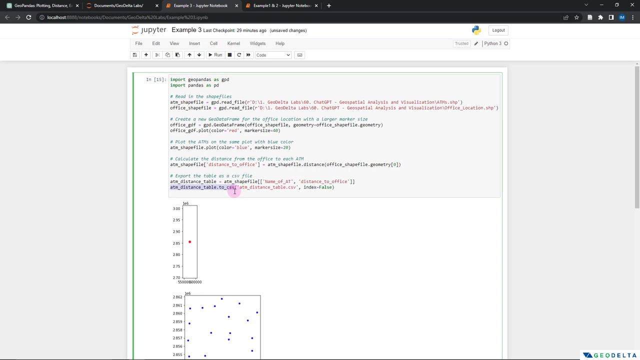 And I would definitely like to keep this distance to office column as well, because that way I would be able to see directly what is the distance between each ATM and this ABC electronics office location. And finally, this line of code would export that to a CSV file. 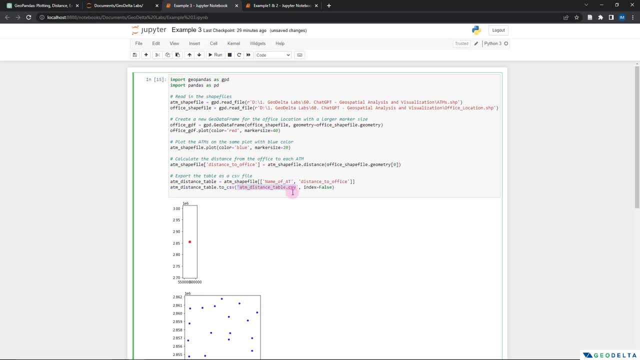 And if I don't really specify the entire path, this file will get exported to the location where we save our Jupyter notebook. However, if you were to add your own path, you could also save it to a different location. So if you were to add your own path, you could. 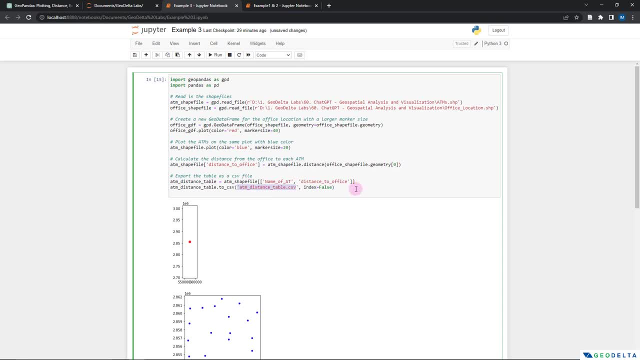 save it to a different location. However, if you were to add your own path, you could save it to a different location. So if you were to add your own path, you could actually export the CSV into a folder location of your own, And over here it's basically deactivating the index, which we don't. 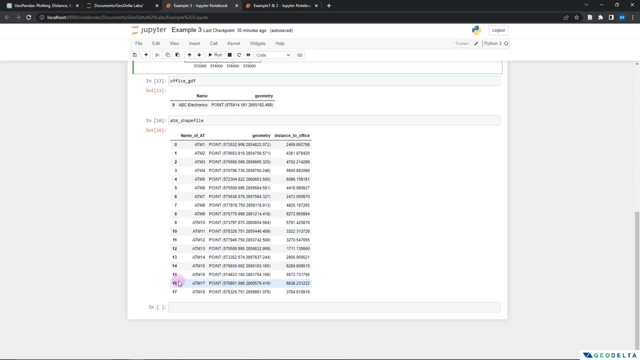 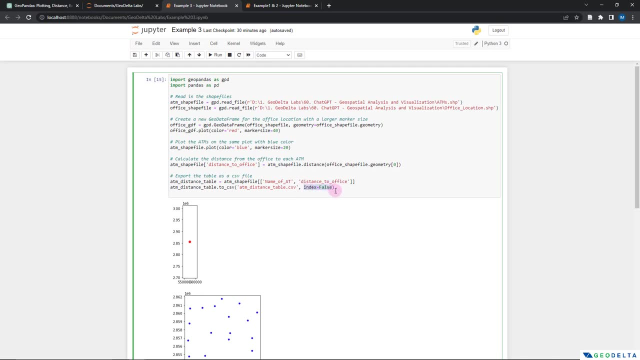 really need. However, for some reason, if you would like to still retain this index column, you can leave this index argument to be true, But if you specify the index argument to be false, that'll sort of disappear in the exported file. Alright, now let's execute this command. 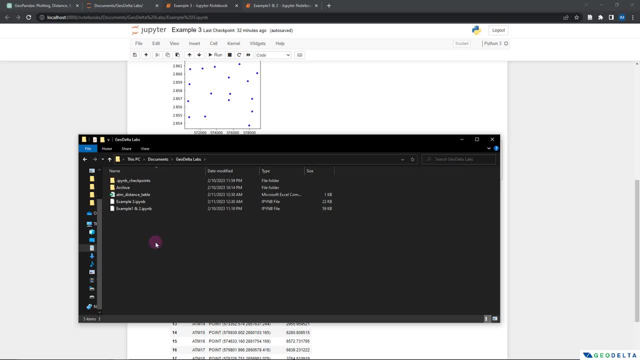 If I head to the folder where I have saved this- Jupyter notebooks- you can see that this file basically got created: ATM underscore, distance underscore table. So let's just go ahead and open that up And, as I told you guys, you can see that this index column. 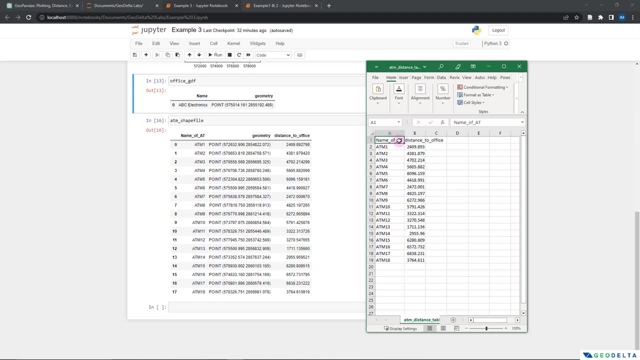 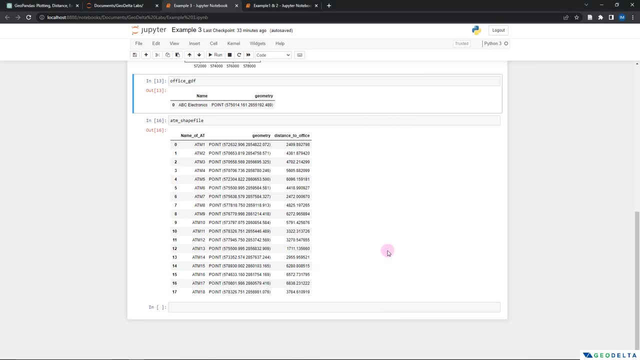 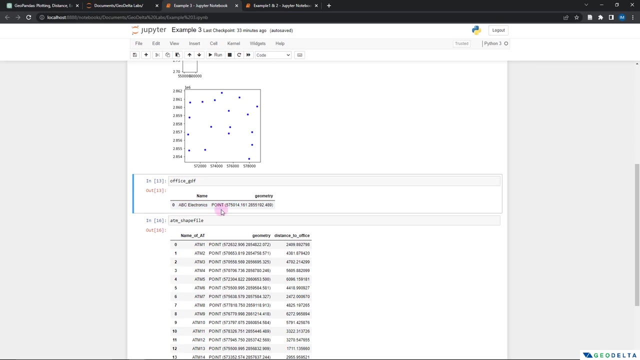 no longer exists. Instead, what we have is this name of ATM and the distance to the office as well. Pretty cool, isn't it? So before I wrap up this tutorial, I would like to sort of extend this example three by specifying a case where we have two office locations instead of just one. 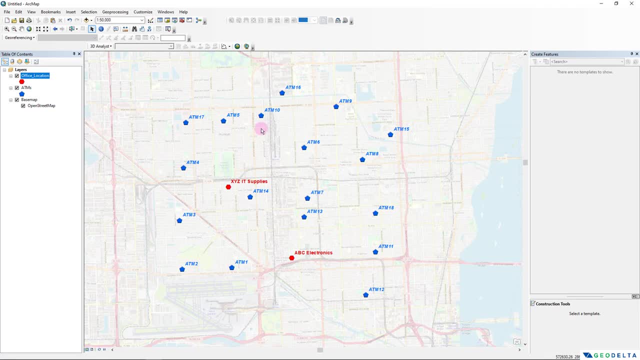 And if I were to visually show you guys how such a case would look? this is how it would potentially look. So you can remember that in the previous example there was just one location called ABC electronics, But now you can see that it has two different locations. If you were to explore the 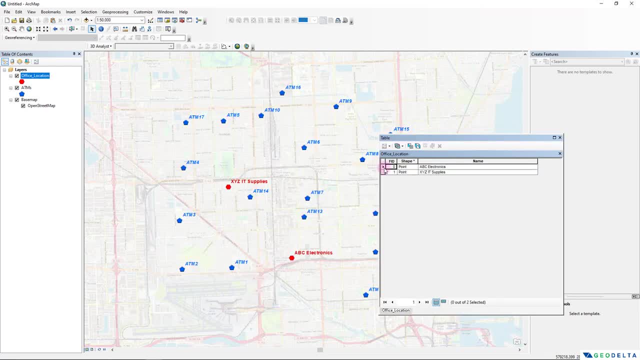 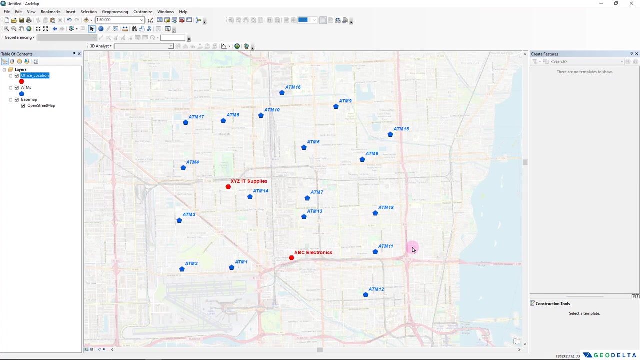 attributes table. you can see that now we have two different features, just like this: ABC electronics, and another feature called XYZ, IT supplies. So what we can do is we can actually advise ChatGPT on this new circumstance and see what sort of a response we can get when it comes. 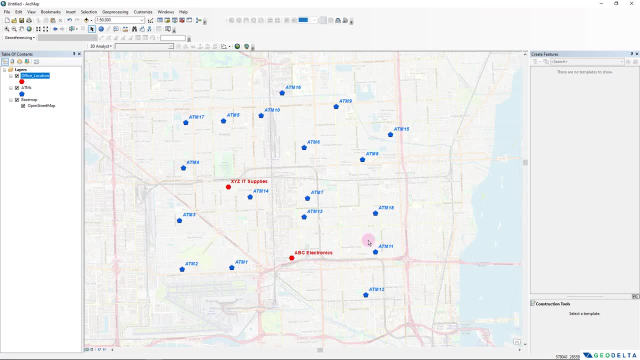 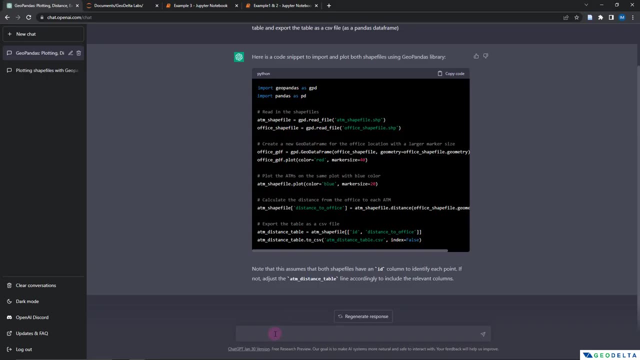 to doing the same sort of an operation in calculating the distances between the locations of the two offices with respect to the location of each ATM. So what I can do is I can head back to ChatGPT and say: what if the office shapefile contains two features instead of just one? 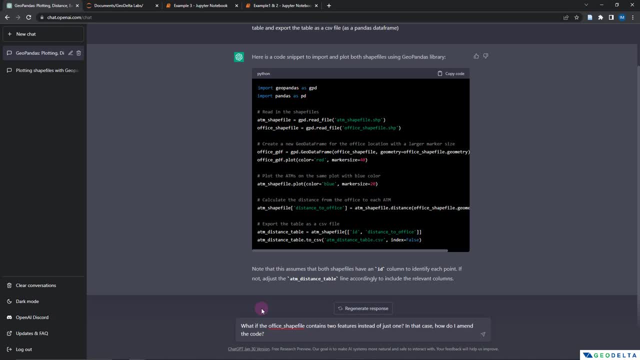 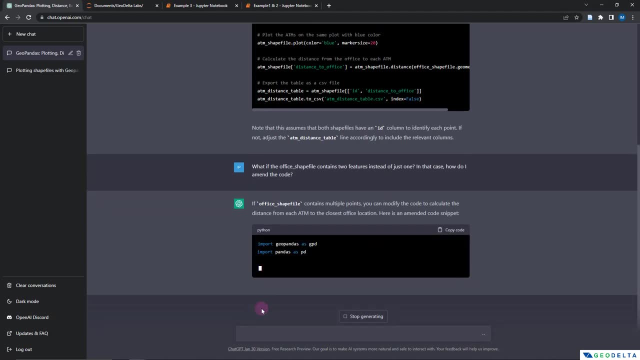 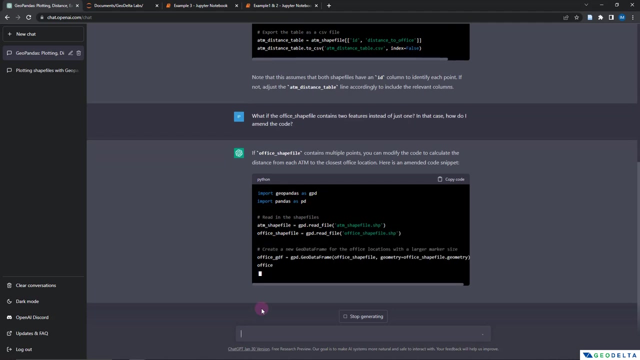 In that case, how do I amend the code? Let's just pass this sort of a request and see what kind of response we are going to get. Well, it's saying that if office shapefile contains multiple points, you can modify the code to calculate the distance from each ATM to the closest office location. 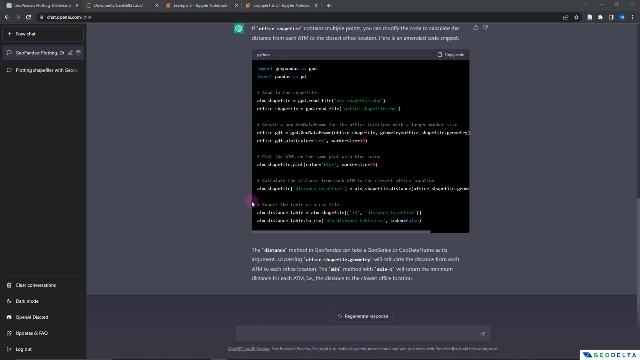 Well, in this case, what it's doing is it's basically finding out the closest office location. So I think we might have to be a bit more descriptive when it comes to our request, because what I would like to do is, in the final table, have three different columns. 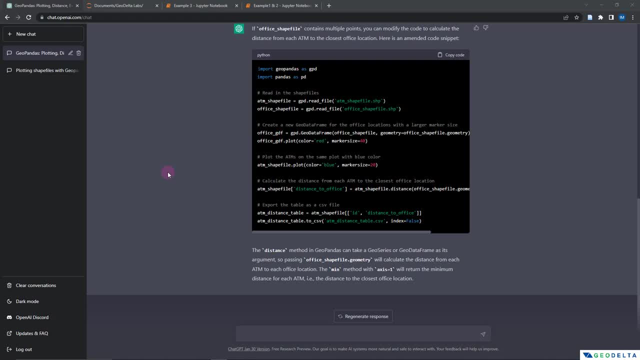 And the first column obviously can be the name of the ATM or the ATM ID, And the second and third columns should basically tell me the distances between the offices and the ATMs separately. So let's just refresh this request a bit to be a bit more specific. Alright, so I have. 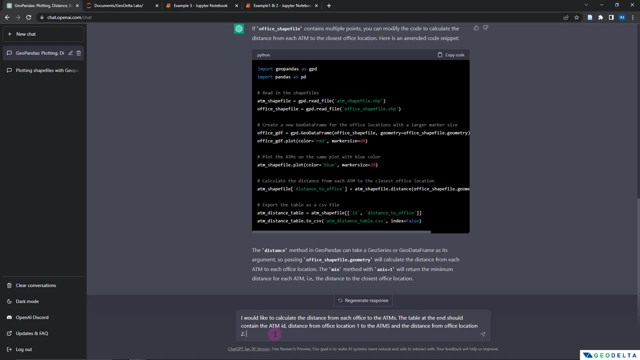 rephrased my request. I would like to calculate the distance from each office to the ATMs. The table at the end should contain the ATM ID distance from office location one to the ATMs and the distance from office location two to the ATMs. Alright, let's hit enter and see what sort of a response we get. 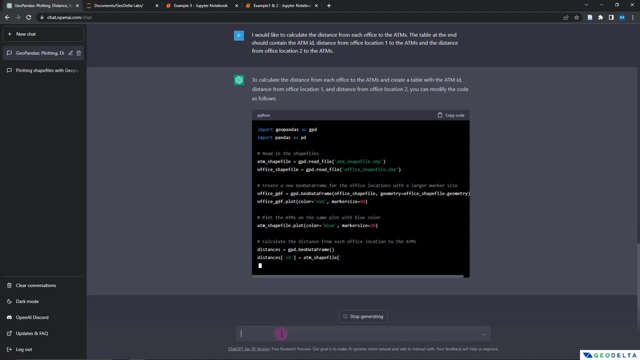 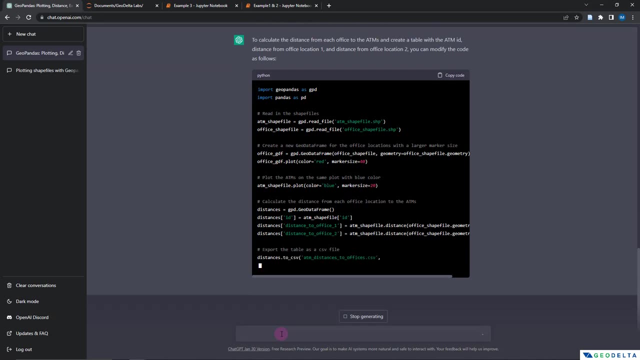 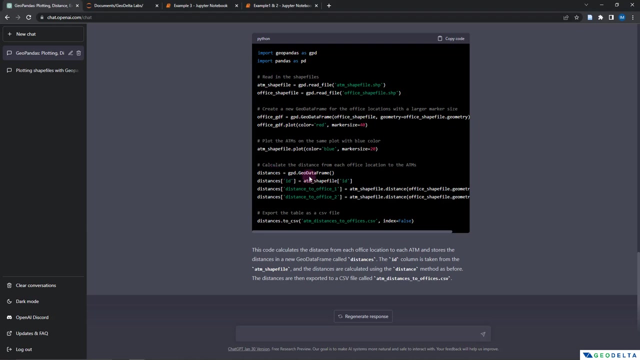 So you can see, I have created a new geopanda geodata frame which is called distances and basically sliding in the information of the ATMs as well as the distances corresponding to office one as well as office two. So what I'm going to do is I'm going to basically 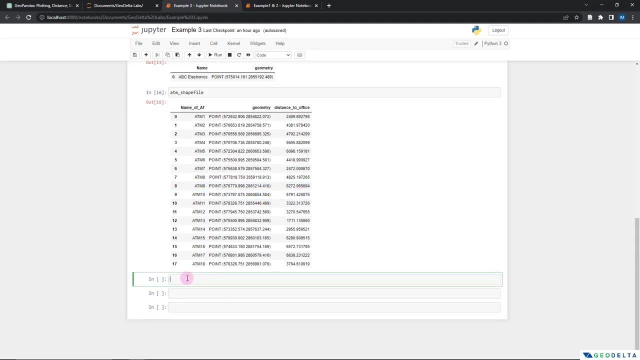 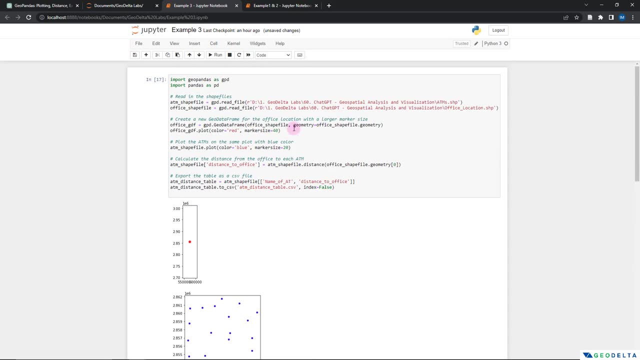 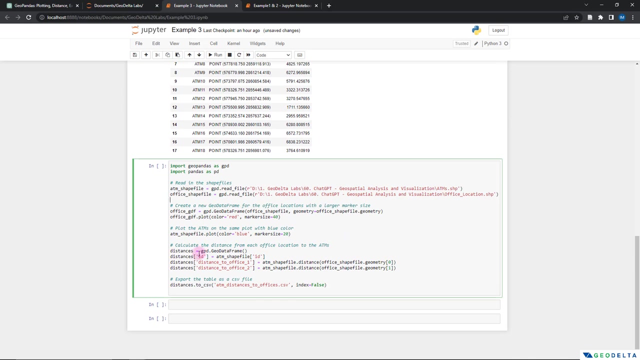 basically copy this code, snippet and paste it, maybe in a new cell, And we can get rid of this and sort of slide this part in like this. And, as I mentioned to you guys, what it's doing is basically it's creating a new geopandas geodata. 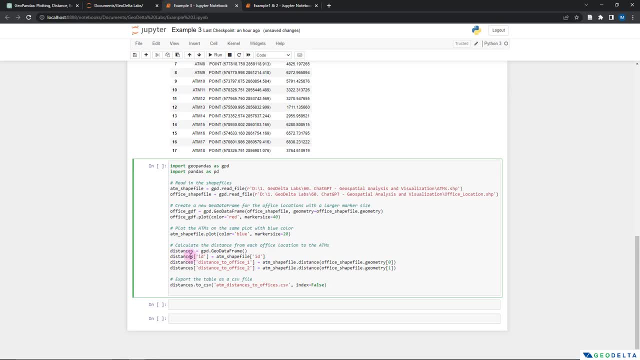 frame, an empty geopandas geodata frame called distances, And into that distances geopandas geodata frame. it's first assigning a new column ID called ID, And in the example code what it's basically looking for is the ID of the ATM And 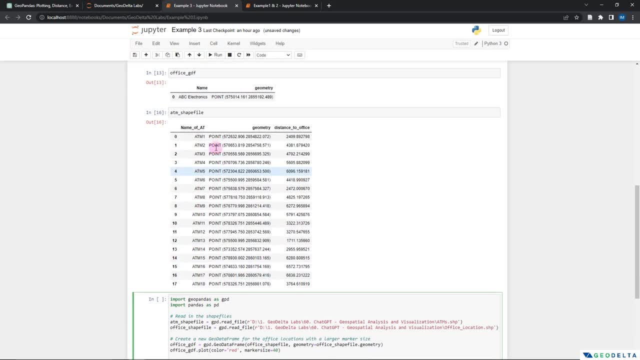 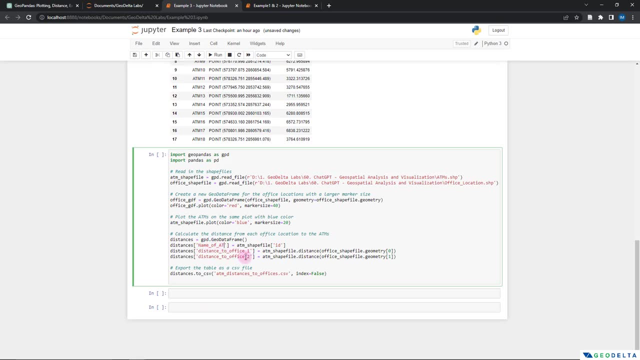 since we know that we don't really have a column name called ID, but instead we have one called name of AT, which is giving us the name of the ATM, we can simply slide that in as well, And in addition to that, it's also adding two. 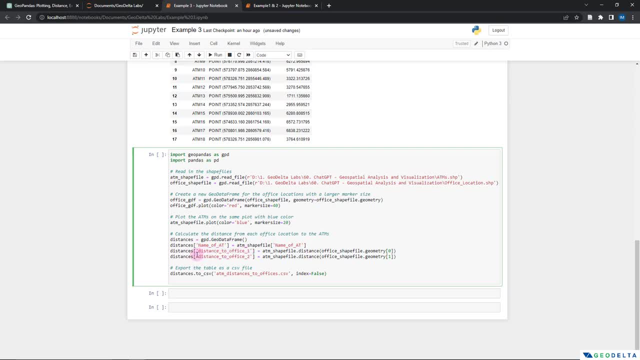 more columns, The first column called distance to office one and the second column called distance office two. And when it comes to referring to the geometry element, you can see that for the distance to office one, it's searching the distances from each ATM location to this zero element which basically gives the location of 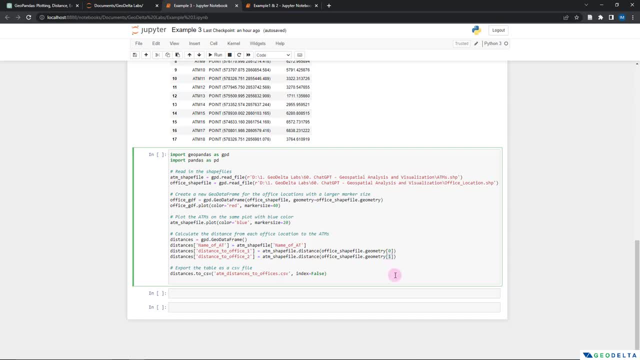 the first office. So this is basically the item at index number one of the office shapefile And that's going to be the information of office number two And with respect to that, it's doing the calculation of the distances of each of the different ATM locations. So what we can do is we can basically execute. 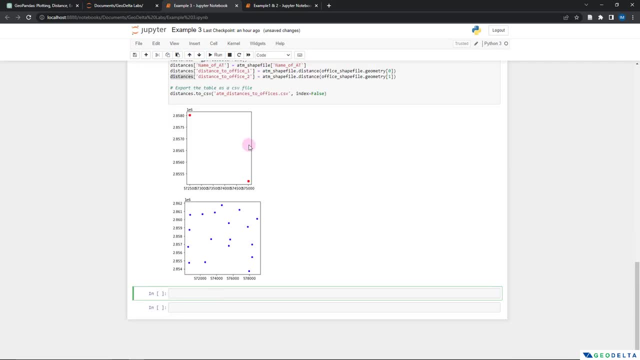 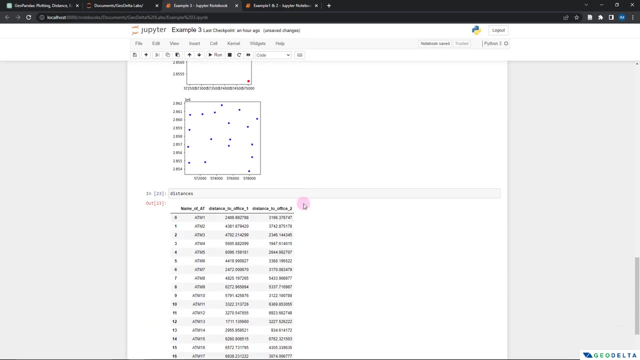 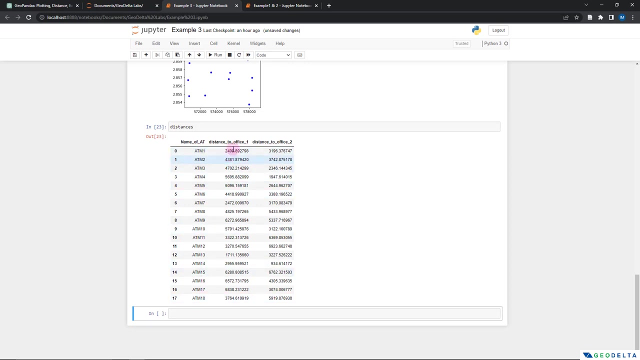 this code snippet And I would be interested to see how these distances, geopandas, geodata frame look. So let's run this cell And over here you can see that. now what we have is basically three different columns: the first column showing the ATM ID, and the second and the third column showing the ID of the 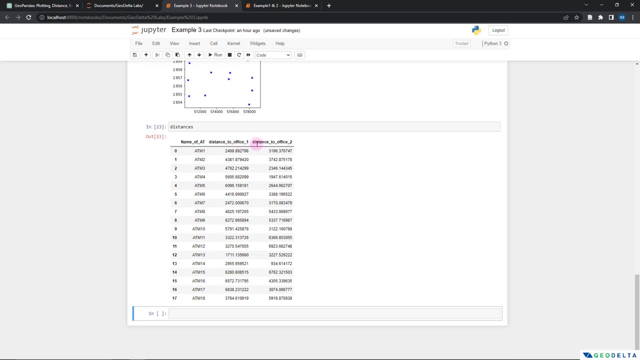 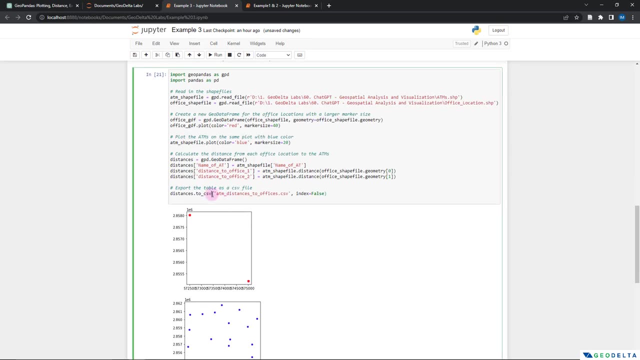 ATM And the third column is basically showing the distance to office one and distance office two from each of these different ATMs. And if we head back to our original folder, yeah, we would be able to see this: new ATM distances to offices- CSV. 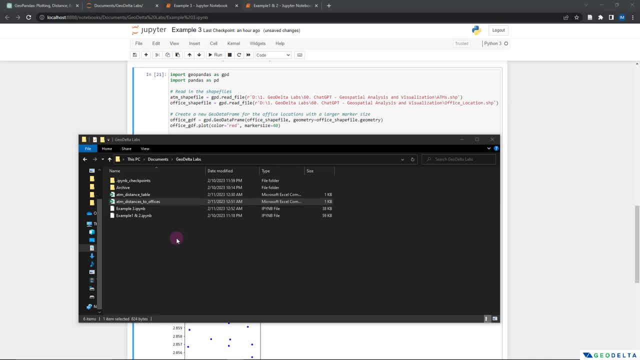 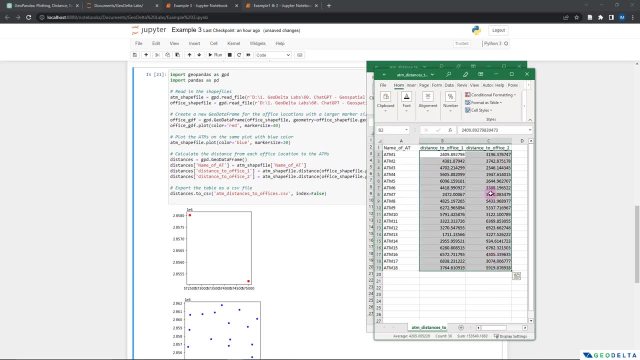 file as well. Let's go ahead and open that up And this is how that file basically supposed to look. We have the three columns and the distance information, just like this. So pretty handy in getting stuff done using chat GPT, isn't it So, as you can see, in certain cases it's. 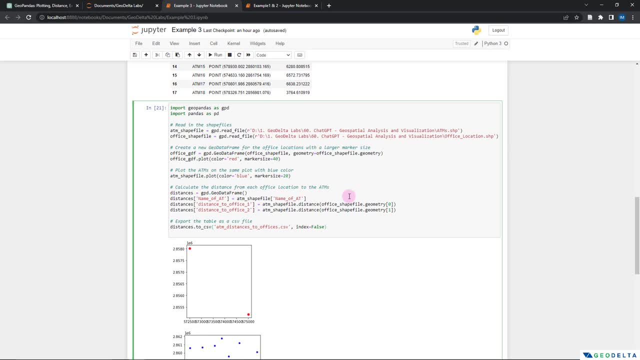 still going to need some human input. it's not able to do everything completely by itself, So that's why this is going to be a good tool that kind of elevates your productivity. if you have some sort of a base knowledge And if that's the case, if you know exactly what to search for, this is just going to 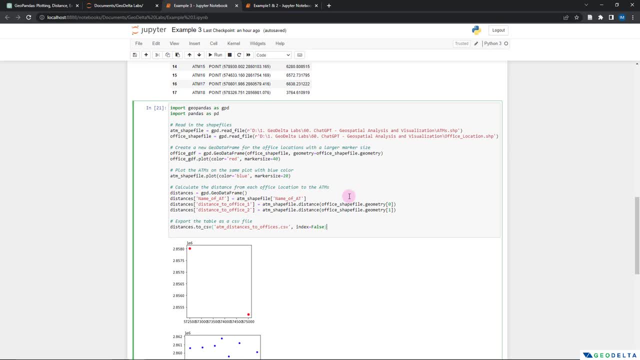 boost your productivity exponentially, I would say, which can make your life much, much easier by being able to get stuff done without having to read through lots of information If you were to just browse the internet in the traditional way. Alright, guys, so that concludes the 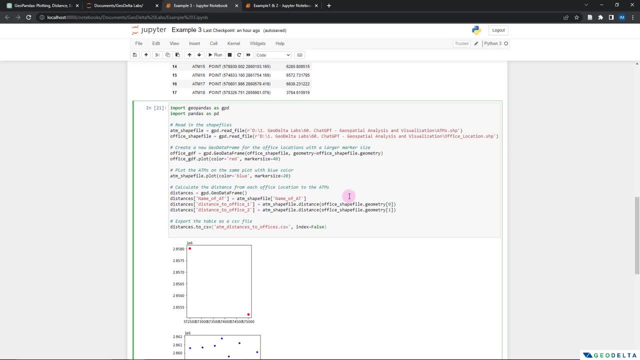 example number three. And now we'll head to example number four and see what sort of a geospatial analysis we are going to talk about in example number four in the next part of the tutorial.